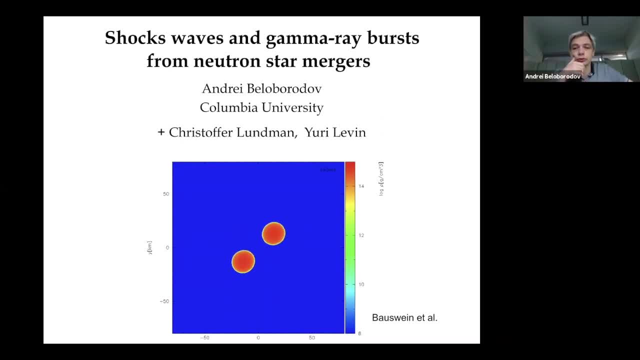 theoretical simulations of neutron star mergers and how they would produce. you know how the two stars would dance around each other, then merge, produce gravitational waves, Also produce a cloud of radioactive material that can emit optical light, synthesize heavy elements And also for many years it was speculated that 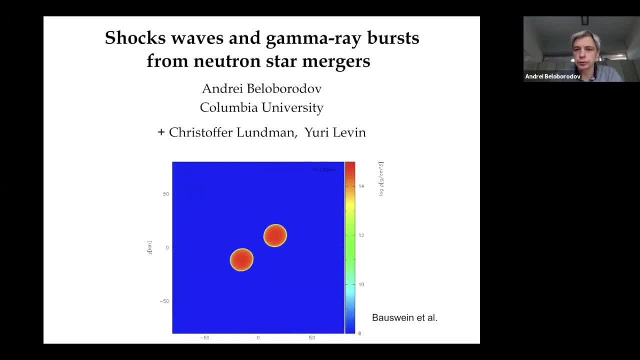 this kind of events would produce gamma ray bursts, short gamma ray bursts, And three years ago there was a first neutron star merger detected where all these components actually observed both gravitational waves and gamma ray bursts, And I'll talk a little bit about this in a bit. 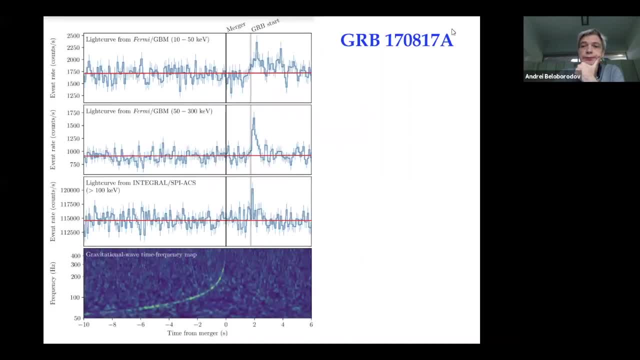 So this is the gamma reversed and the gravitational wave picture that I'm sure you've seen before. So the bottom panel is the chirping gravitational wave signal- Our frequency goes up with time- And the three panels above it are the light curves of the gamma reverse that accompanied that event in three channels between 10 and 50 kV, 50 and 300 kV, and you see about 100 kV in the real data. 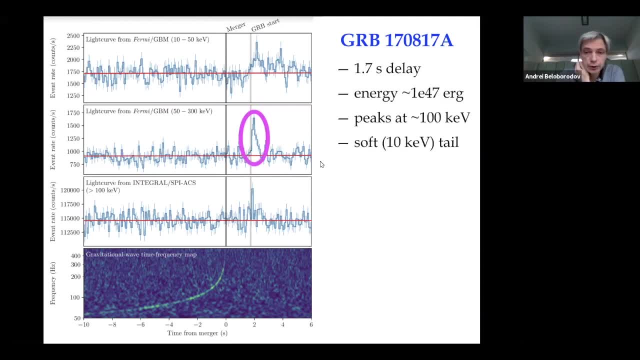 And so what you do see here is the is the is the is a nice spike, strong spike of gamma rays, which peaks at around, roughly speaking, 100 kV, And when you analyze the data more carefully, you find that it was. 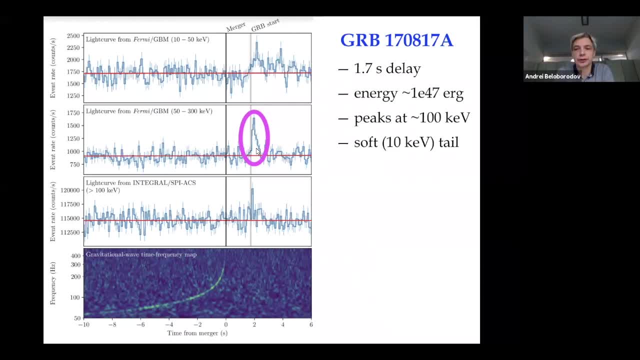 well, first of all, you see that it was delayed by about two seconds relative to the gravitational wave signal. Then you see that this spike was relatively narrow even compared to the delay about three seconds. So it's about three times narrow. 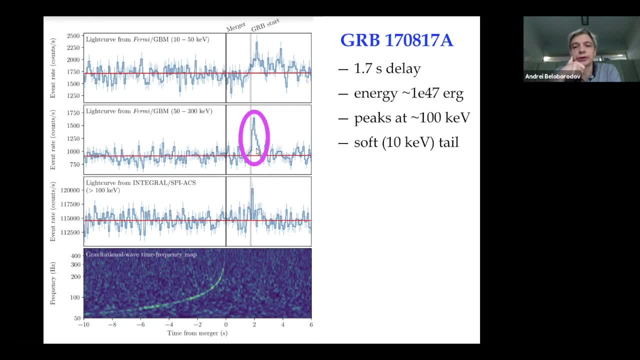 Delta T over T is about one-third. And then, when you analyze the data, you also find that it was followed by soft quasi-blackbody emission. Now it's hard. the data is not so great. it's hard to see what was exactly blackbody. 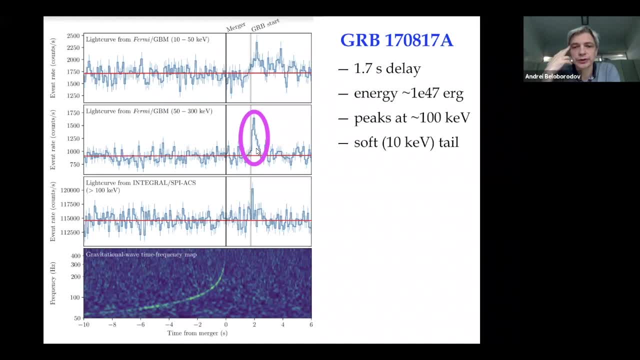 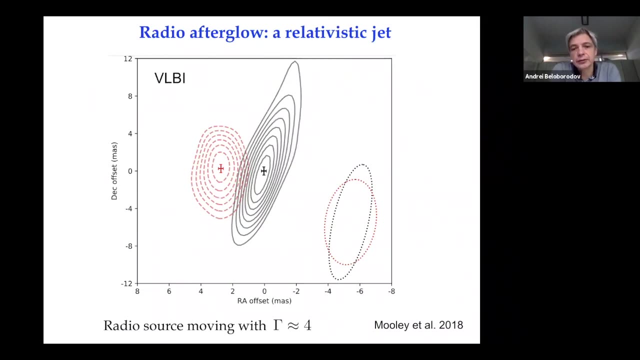 but it was soft emission picking from 20, with temperature about 20 kV, which followed immediately at three, four seconds. Okay, Then what we saw was a clear sign of relativistic ejecta. So in radio imaging just you can see that there was something moving with the range factor of four. 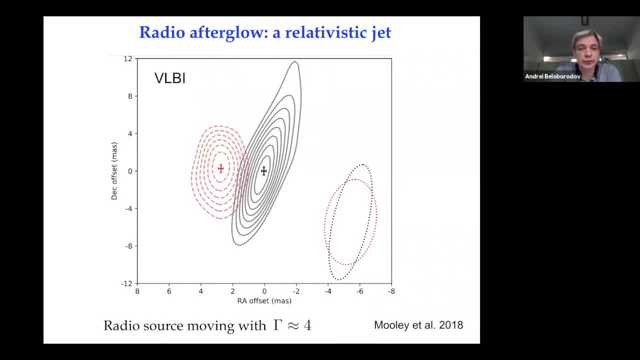 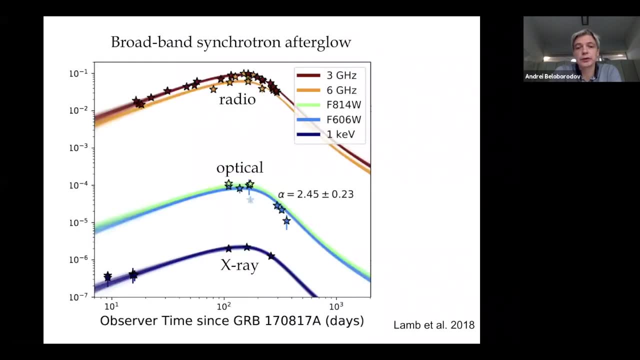 at late time of radio afterglow from that burst. So there is no question that it was relativistic ejecta produced by this event, as expected, You know, in the cumulus burst context before, And there was this broadband synchronic afterglow. 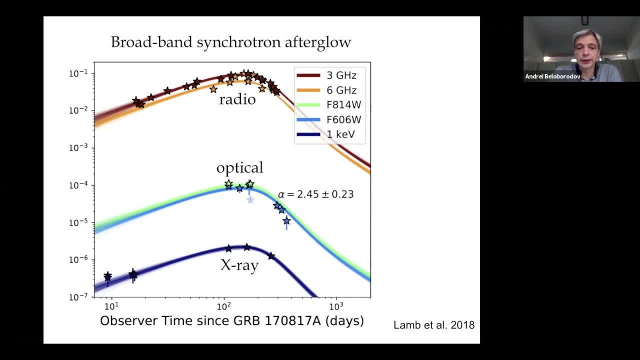 radio, optical, X-ray, beautiful data peaking, as you see here, like a hundred hundreds of days. So, of course, many people- there's many hundreds of papers- immediately jumped onto this data and simulated them different models. 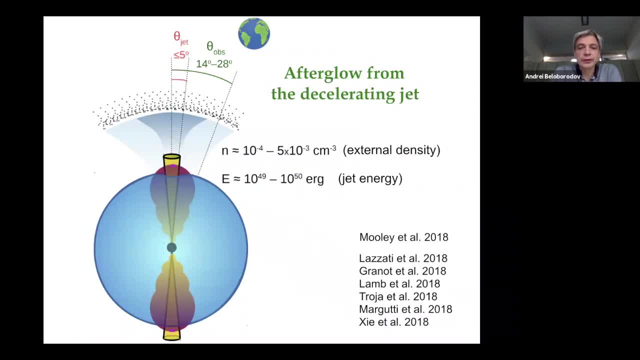 I don't know tens of models, But quickly there was some convergence to basically this picture that what you see is a jet which was narrow, with opening angle about five degrees, As we know from the gravitational wave data, the observer angle with respect to the axis of rotation of the merging binary. 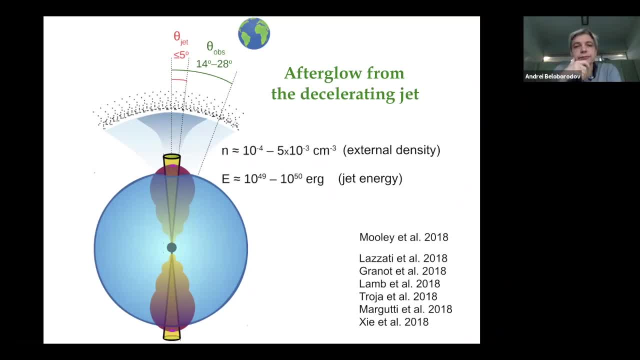 was between 20 and 30 degrees And so basically, during the afterglow phase, you see a narrow jet observed off axis And from this modeling of synchronic broadband emission people try to reconstruct the in the density of like in the environment around this emerging binary. 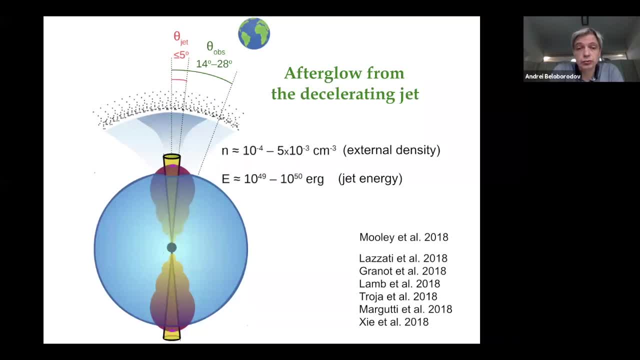 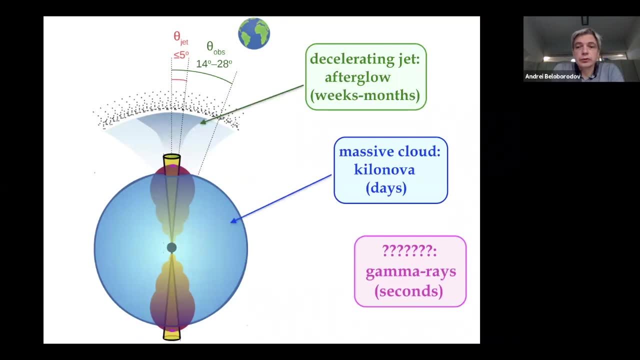 and total energy of the jet, which is 10 to the 50 york. Okay, And so it all came to this basic picture that we more or less understand what it was: a decelerating jet produced afterglow. 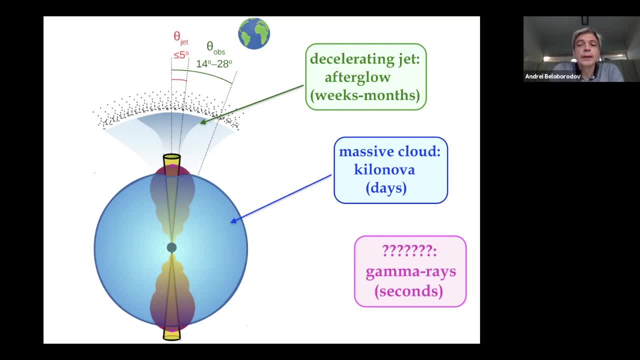 scales of weeks, months, years. There was this massive cloud that produced what we call kilonova macro nova on timescale of days, and it picked an optical infrared and it was clearly signature of radioactivity elements being synthesized. 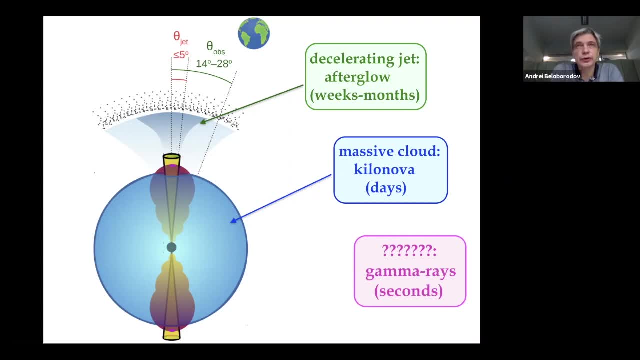 our process, in particular in the massive cloud with a mass of about 5% of the solar mass moving with, expanding with mild, realistic speed, few tenths of C, this heavy cloud, And so the real puzzle that remains. 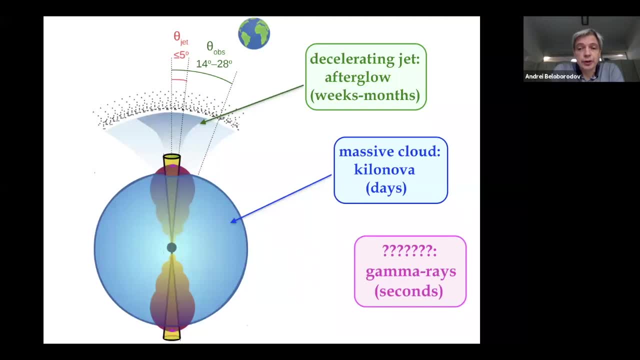 is how gamma rays were produced, how this gamma ray burst was emitted, And I should mention that, since I worked in this field for some years before this detection, so I remember very well how no one actually expected to see anything interesting in gamma rays. 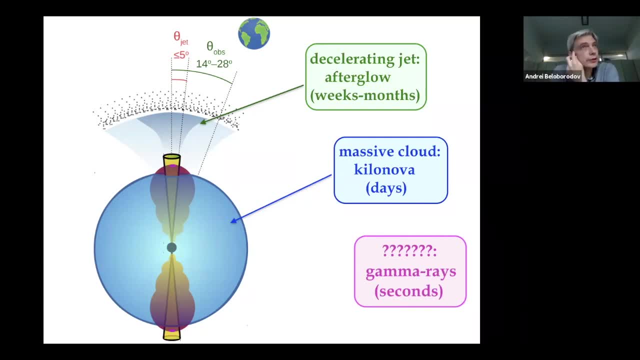 financing non-vibe. Most people would tell you that if you look at the gamma ray burst source off axis at 20, 30 degrees, you probably wouldn't expect to see gamma rays. because this outflow because as soon as you go outside. 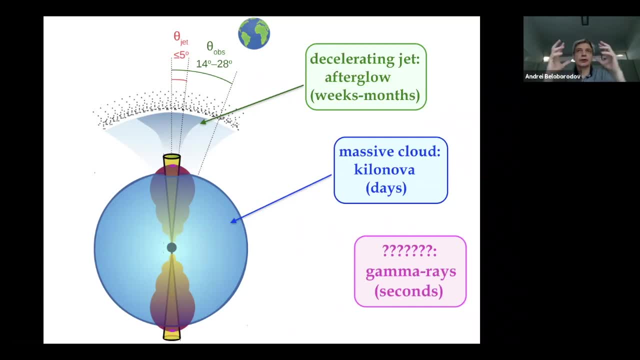 the beam angle of the jet, you expect slow material and whatever you the models that have been done, like hydrodynamical simulations or jet breakout, et cetera, you expect to see emission that was reprocessed to x-rays. 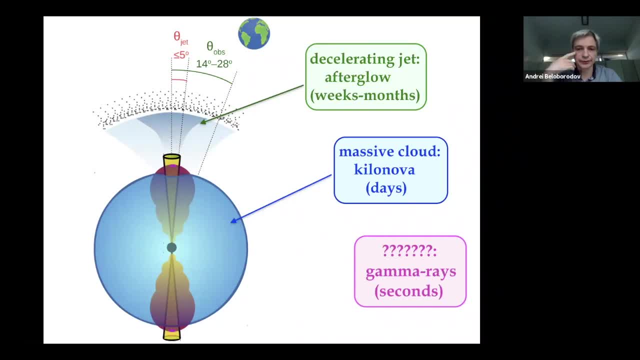 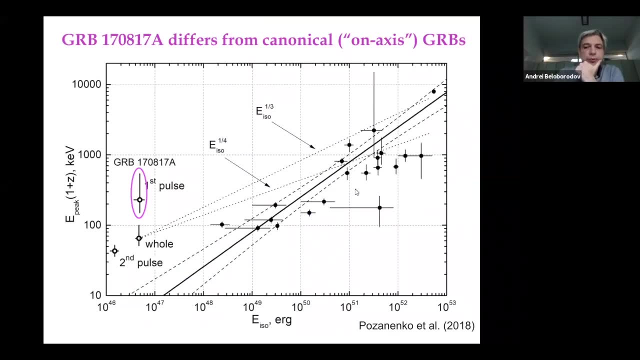 maybe even soft x-ray, but not in gamma rays, And indeed the burst that we see is is strange compared to the the other GRBs that we've seen before. So in this plot you see many GRBs associated. this is short gamma ray burst. 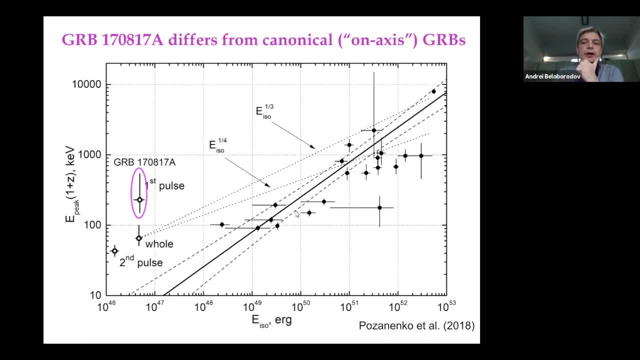 classified as short duration, short heart. This is the class that was associated for many years with Newton's time mergers, And when we actually saw a Newton's time merger, the burst that we see was off axis, but it was. 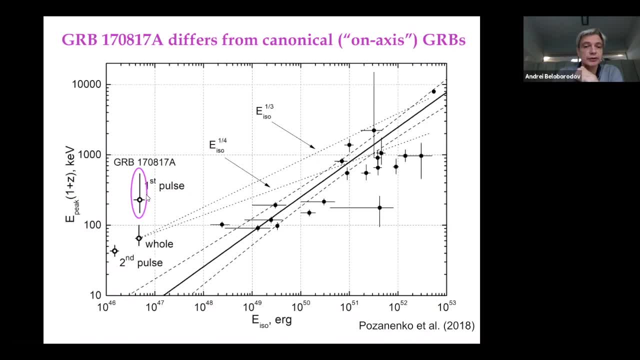 it was weak, as expected, but was very hard, As you can see here. this GRB 1708, 1708, is the counterpart of the gravitational wave event. It's 200 KV roughly speaking. Well, if you extend the correlation of the observed GRB, 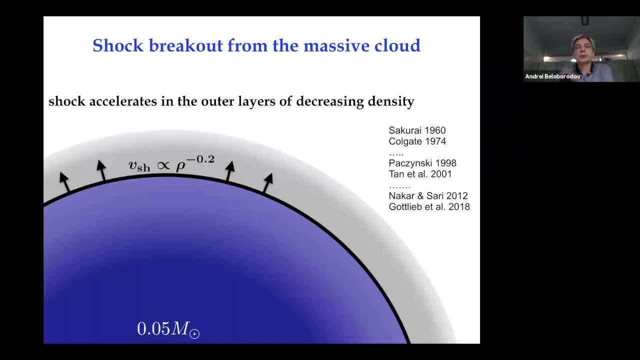 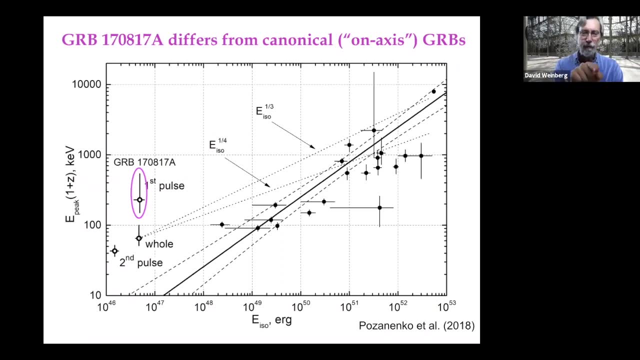 it should be much, much simpler, All right. And so can I ask, go ahead This, this estimate of of 20 degrees, whatever off axis, is that coming from this? or or the estimate of of off axis was coming from? 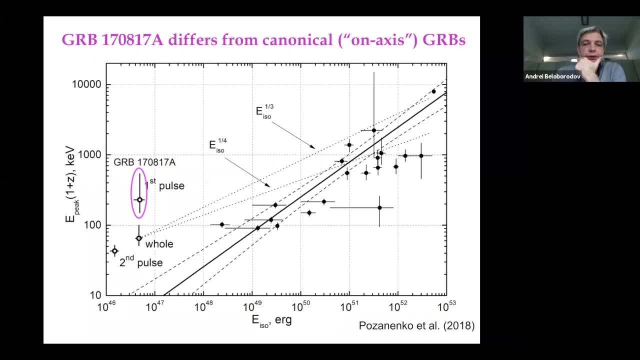 from something else, From gravitational wave data. There was a. yeah, just by analyzing gravitation, how the two stars merge and what kind of gravitational wave, the waveform that you receive, You can already estimate. from gravitational data alone, you can estimate the observer angle. 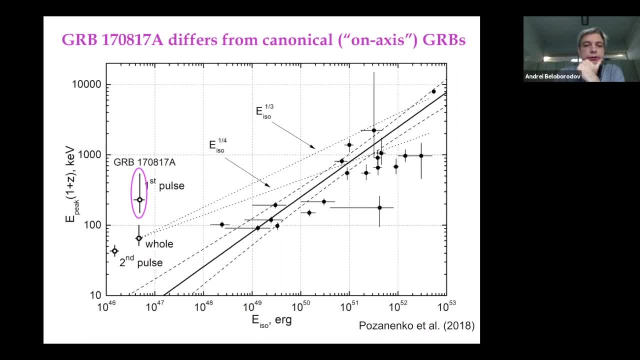 in respect to the rotation axis, And it's about 20 degrees. There is a significant uncertainty, but it's this kind of number: 20,, 30 degrees. Okay, Thank you. That's consistent with the analysis of afterglow. 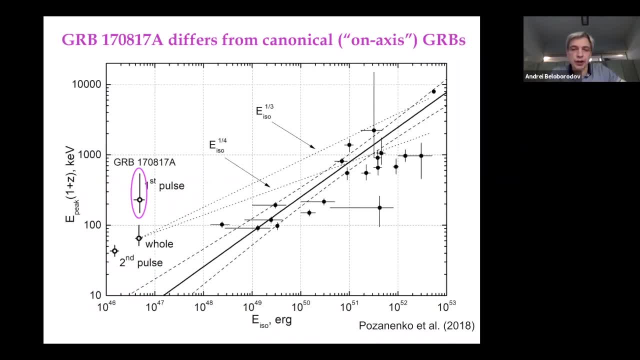 which, which, which came from a jet which initially you see the jet with the delay, for a simple reason: If I go back to the afterglow, my short discussion of afterglow, when you see a collimated jet, 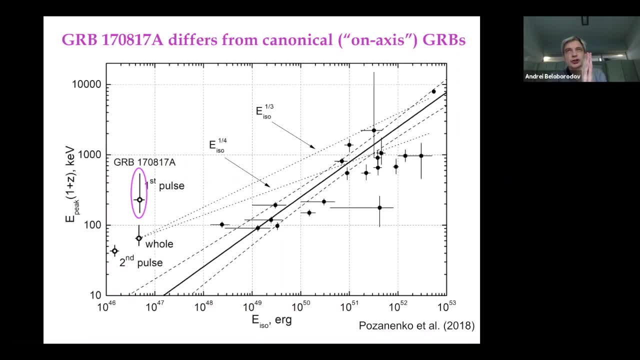 when you look at the collimation at the collimated jet off axis, initially you don't see much because all the emission it produces is beamed with a narrow angle. But later, as the jet decelerates, this Doppler beaming becomes less efficient. 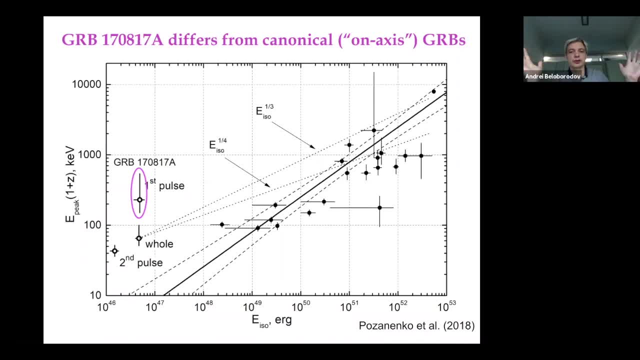 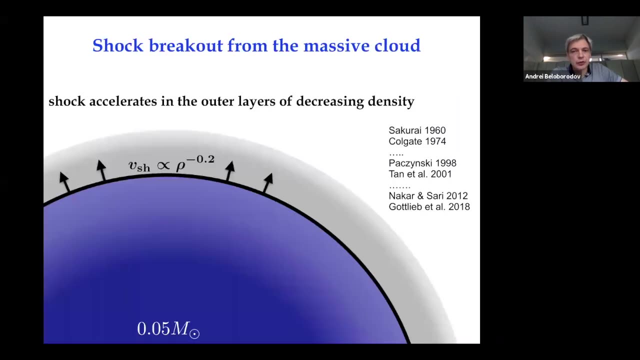 and you start to see broader angle, essentially, And, and then you begin to see the jet, it comes into the line of sight, as it might seem, And that's what's observed there. Okay, So one idea which came. 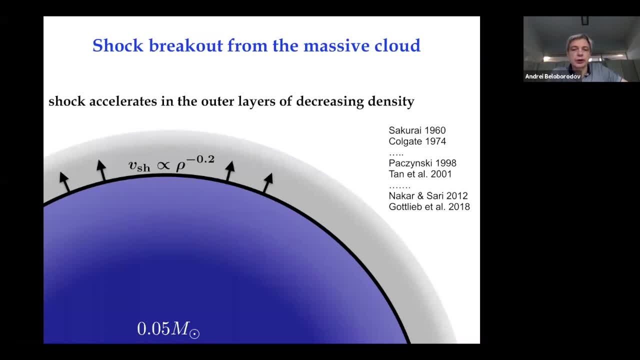 came up immediately is related to the shock breakout picture, which I will talk a little more in a few slides, But the basic idea goes back to like. the basic picture of shock breakout goes back to 50s and 60s. 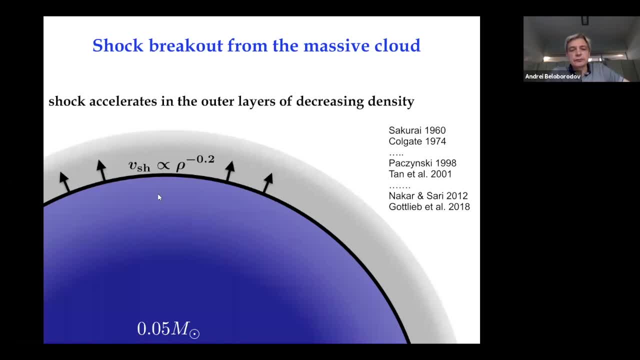 and 70s. So when you, when you have a shock and suppose, in this case, the merger itself, somehow watch the shock and that shock crosses the massive cloud that eventually meets the kilonova, As the shock comes to the edge of the cloud. 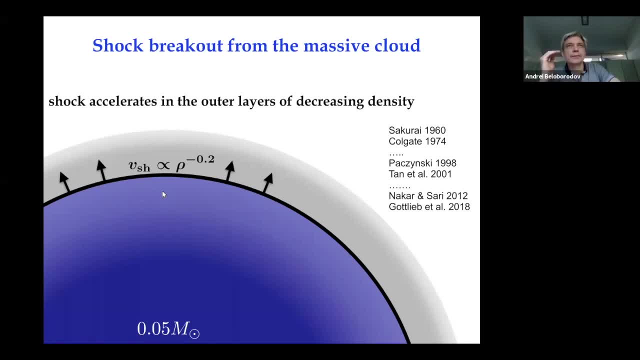 where the density drops it begins to accelerate. So shock dynamics responds to quick decrease, sudden decrease in density by accelerating. So its energy goes down as it goes to lower and lower densities. But energy per particle goes up. 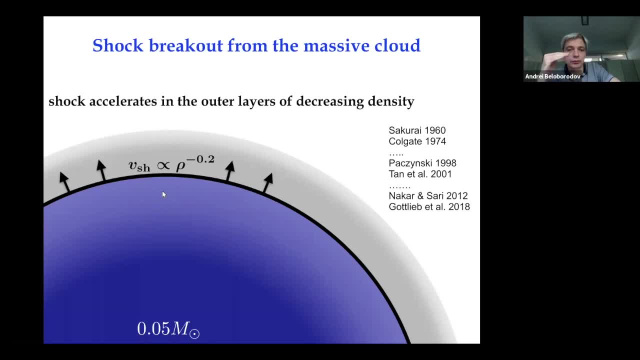 And as a result, the shock. So it's a self similar solution that was obtained first by Sakurai in no relativistic case in 1960.. And you can find discussion in classic academic textbook, For example. 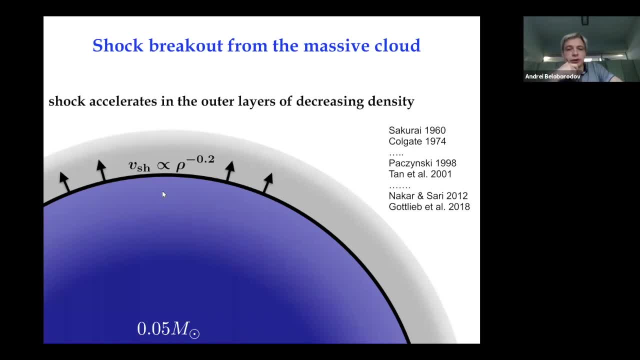 the version Reiser, And so that's a potential source of gamma rays in principle. So from this cloud, if there is a shock breakout, you could see something hot which would potentially meet gamma rays. This idea, though. 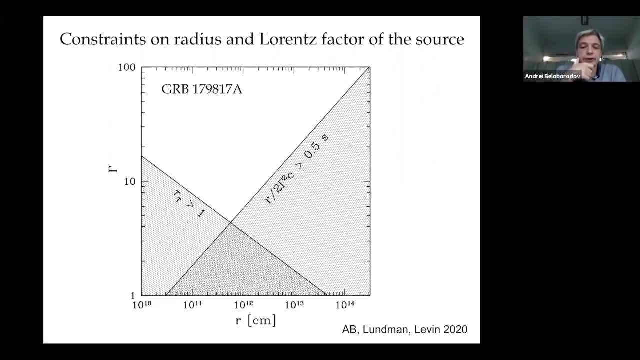 is in tension with- find it quickly. that is in tension with data because in its original form, let's say, Because there are two constraints on this, on this gamma resource that come from the duration of the gamma ray bursts. 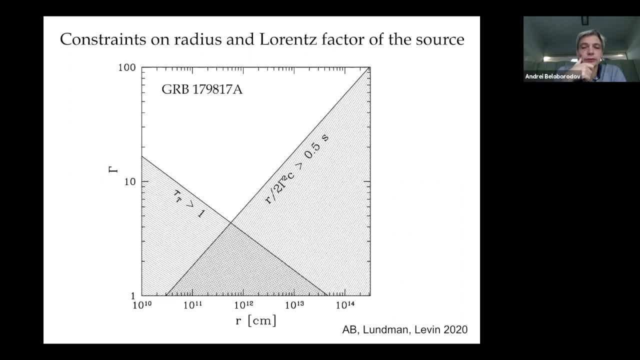 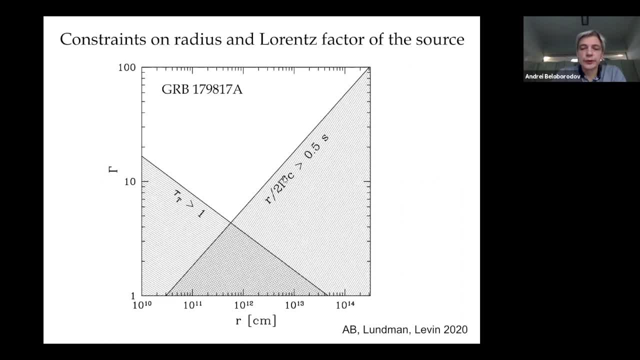 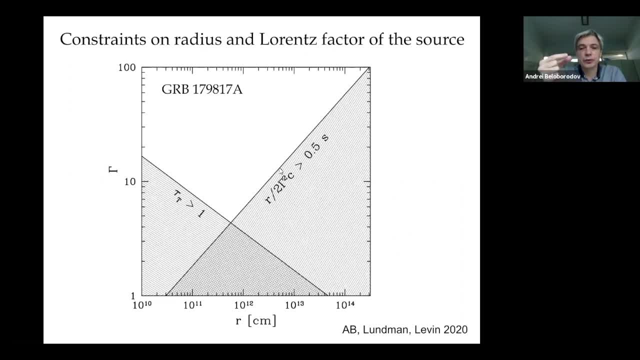 use Doppler compression upon compressed the duration of the burst of the absorbed window. On the other hand, high gamma is also needed to help the gamma rays escape, Because if gamma is too low, then the meeting source. 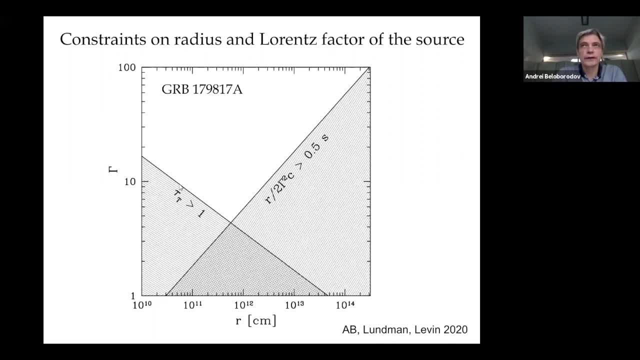 becomes opaque to photons, just to schedule and it's not self-consistent. So these two regions show you, give you the shaded regions are excluded by these two constraints, And so you can see that the minimum gamma here is about five. 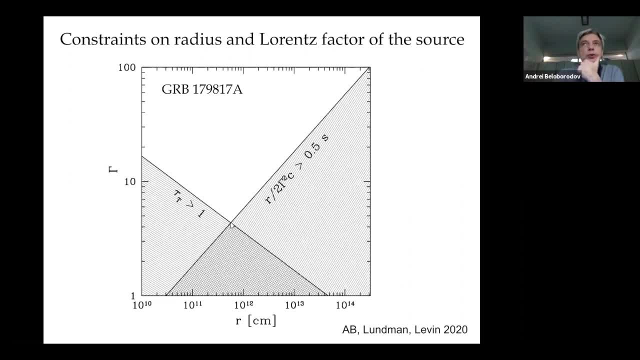 And when you compare it with the shock breakout problem, when shock comes to the edge of a mild relativistic cloud, in that simulation you find that emission comes from gamma is a four-unit to basically mild relativistic. So there is tension there. 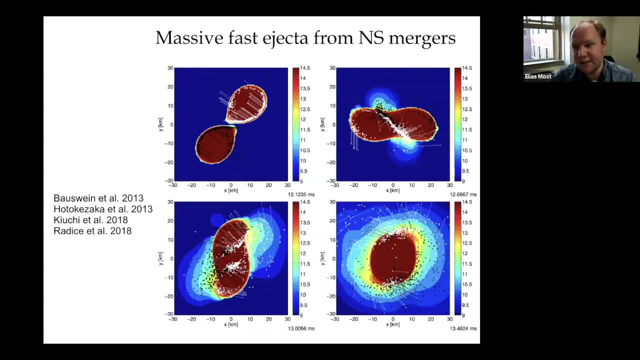 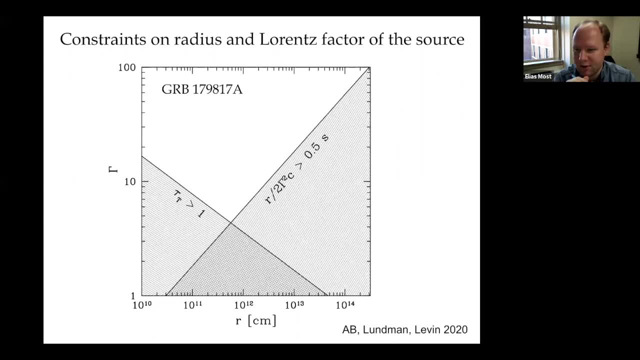 Okay, Andrei, can I ask you a question about that, Like this tau t, like what are the assumptions that you plug in for the density at which at which that happens? Does it just come from the self-similar solution or what do you assume there? 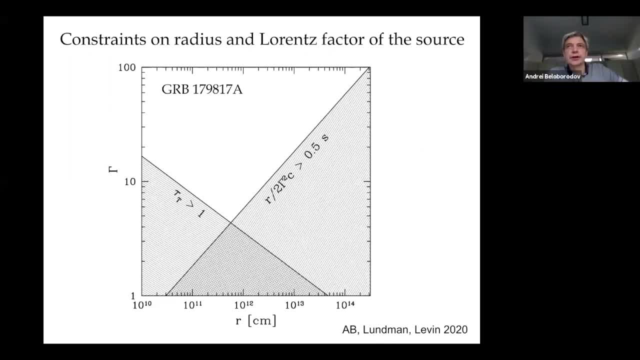 Yeah, So there is a numerical factor that reflects the in the paper which is published, or you can see they're actually a couple of flights- for the optical depth constraints, which have a numerical factor for unity, depending on how the density is stratified to the useful rate. 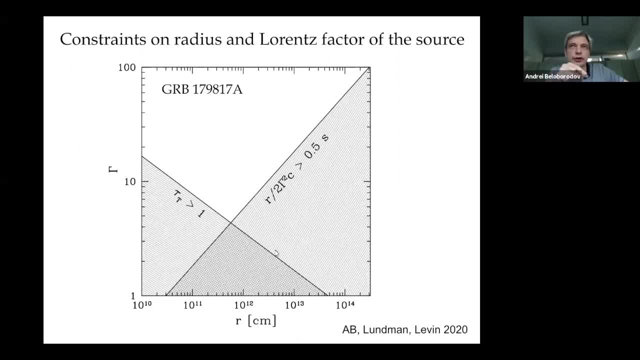 it fairs as by a factor of two or three, But when they translate it, the variation of gamma, it's very small. Okay, Gamma five is the most conservative case. Yep, And of course, when you esteem it, the amount of mass that you have, you, you. 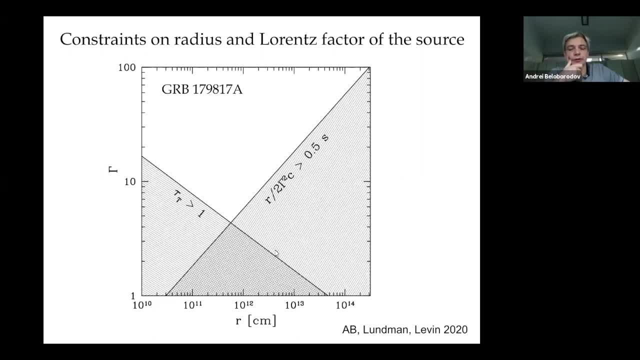 use the energy budget of the Andrey and you said there is a tension here. What is the tension exactly? I mean, you do have a wide, a lot of white space here, A lot of white space, all with high gamma, Yes, and so what's the problem And the 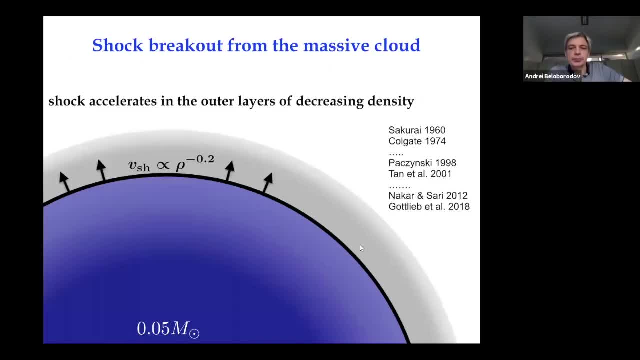 problem is when you look at these papers that I particularly applied to this burst and calculate at which point the shock should be meeting gamma rays, that is, when it becomes transparent, right when it comes to the photosphere. At this point gamma is still like 1.5 or something. It's mildly relativistic. 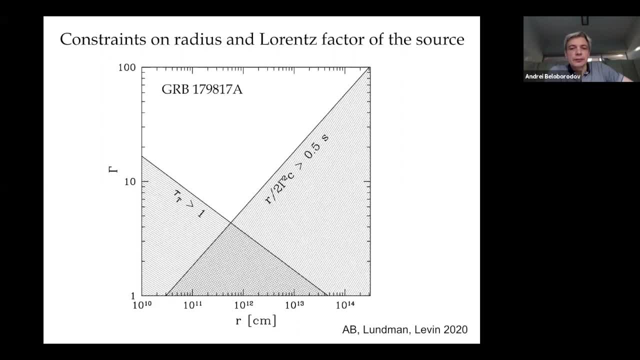 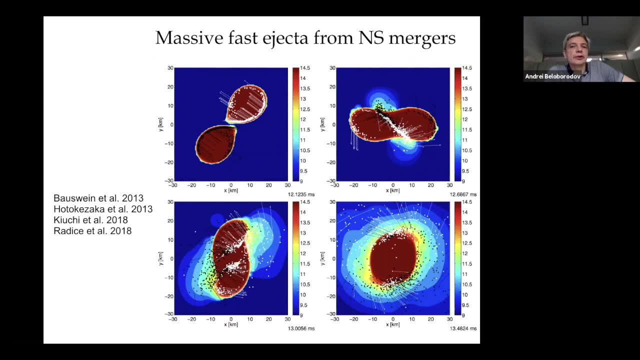 Okay, But okay, but then you can ask question. I mean, okay, how do you know that the Macy projector from Newton star merger? maybe there is fast ejector? Why do they have to have this speed of like a few tenths, mildly? 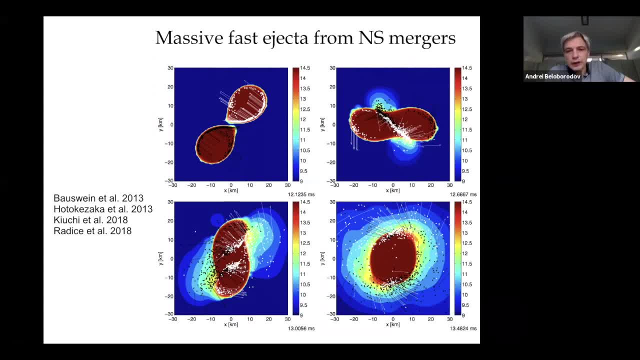 relativistic Speed that we see in the kilonew, And numerical simulations suggest that there is fast material. This is a snapshot from numerical simulations and this white point show the mass elements that will later escape with high velocities, So you can see where they originate. A lot of them originated here at 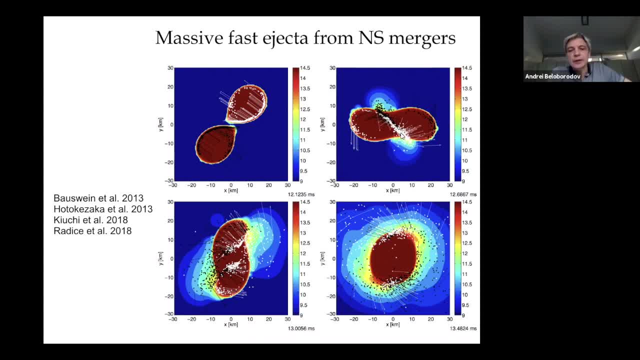 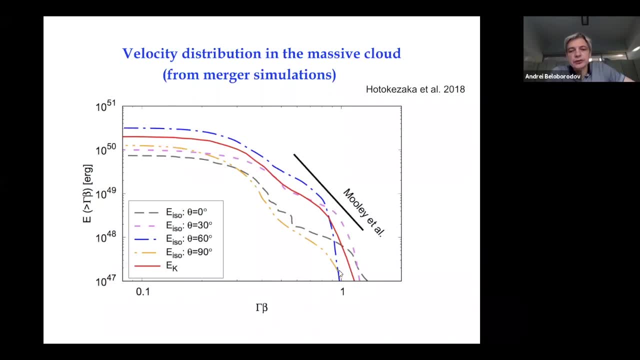 the interface of the colliding Newton stars And you can analyze the distribution of the ejected mass of the gamma better for velocity. And then we still find that there's almost nothing above gamma better for unity. Maybe it goes up to two, certainly not to five. However, I think these simulations have no 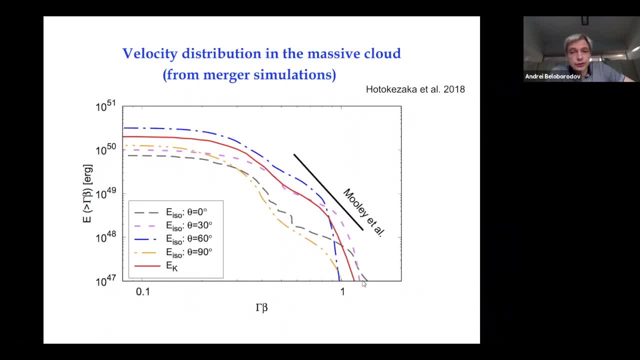 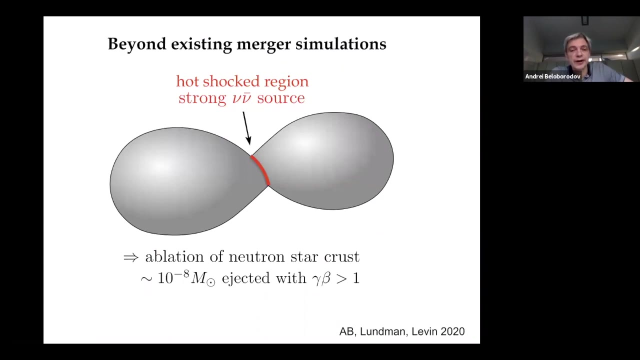 hope, because of their existing resolution, to actually see the fast material that actually exists there. It does move fast And I will just describe why I think the There must be really fast, low mass, fast material ejected by the Newton star merger at the very beginning, Basically once when the 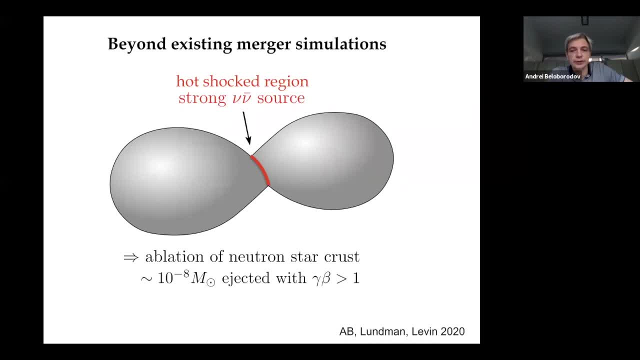 star touching merge in milliseconds. they immediately check low mass, alpha, relativistic and below. So one process. I will mention this briefly, but you can read the paper if you're interested. One process is that when is the ablation? Ablation of Newton star surface by the neutrino emission that is generated? 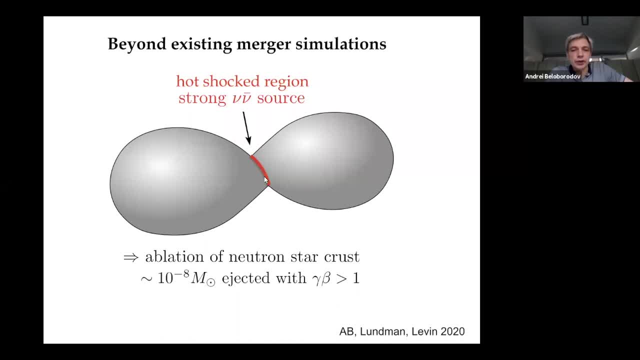 at the interface of the colliding stars. So what happens there? when the two stars touch, they launch a pair of shocks, They create this hot red sandwich with temperature about 20 maybe- And then this is a huge source of neutrinos. And so when these neutrinos, 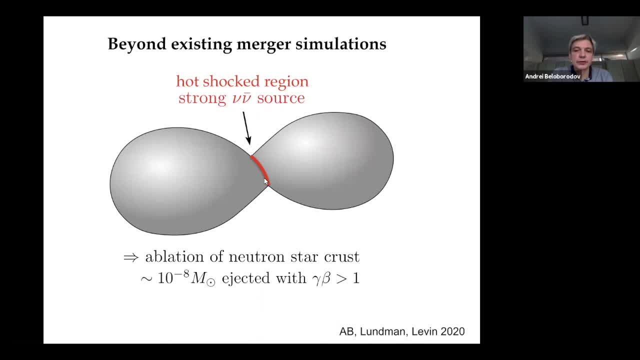 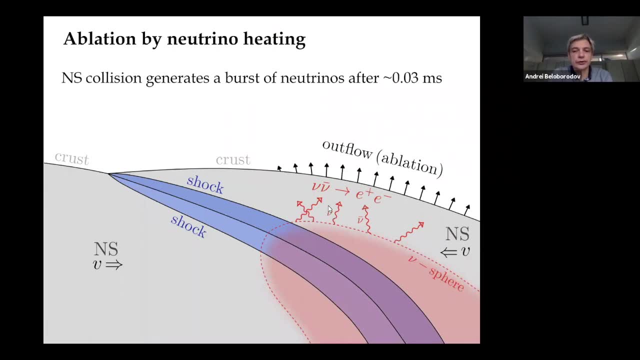 propagate through the stellar material. some of them experience collisions. Neutrinos and antineutrinos collide with each other and turn into electron poisson pairs. So just zoom in on that red region. You see this blue material which is the shock heated material in the 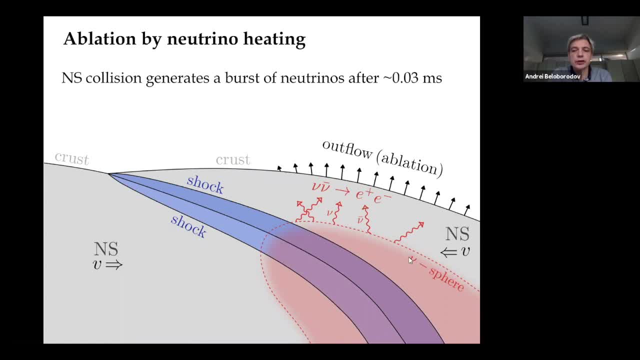 sandwich. You see the neutrino sphere here in red, And then from this neutrino sphere you have neutrinos. You can calculate the flux of neutrinos, you know the temperature of these neutrinos and then you can calculate neutrino-antineutrino annihilation rate, which works everywhere. 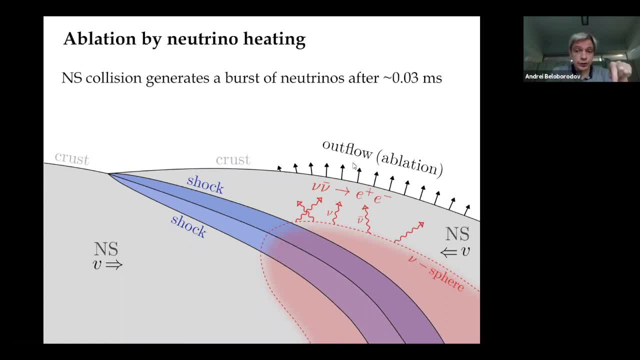 outside the neutrino sphere. So it works here and it works actually even outside, above the Newton star surface. And this annihilation of neutrinos deposit energy in a clean form. They annihilate into electron poisson pairs. So when you look at energy per barrier, like in this region, 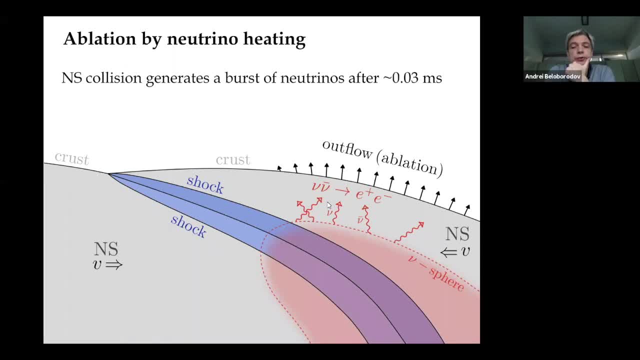 somewhat below the surface. the energy deposit per barrier by neutrinos is not so high because there are lots of barriers In this region. near the surface there are almost no barriers, but neutrino-antineutrino annihilation rate is almost the same, So energy deposit per barrier is huge. 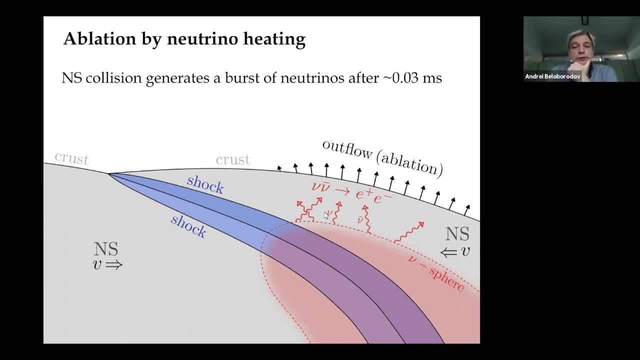 And this neutrino front that goes ahead of the shock wave, the subphotospheric heating that has to ablate the rupto-star surface. So we've done the calculation. It's essentially deposit heat and there is a refection wave, and that's how. 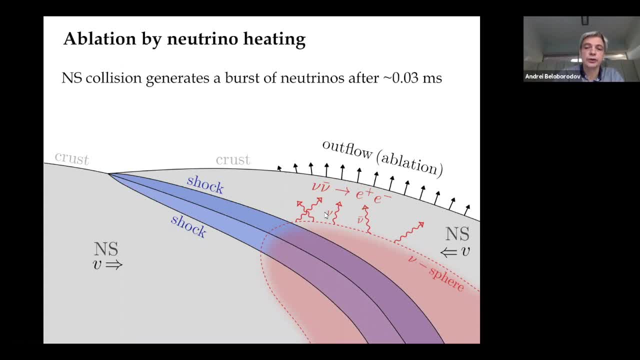 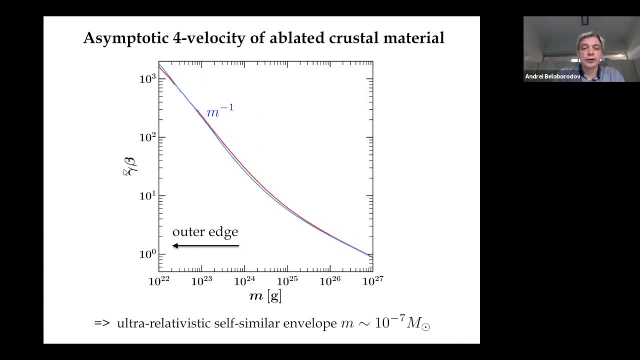 ablation works right. We don't have a limit calculation for that process. and this is the distribution of the ejected material: Lorenz factor for ejected mass and mass counted from the outer edge. So m little m is equal to zero for the first like. 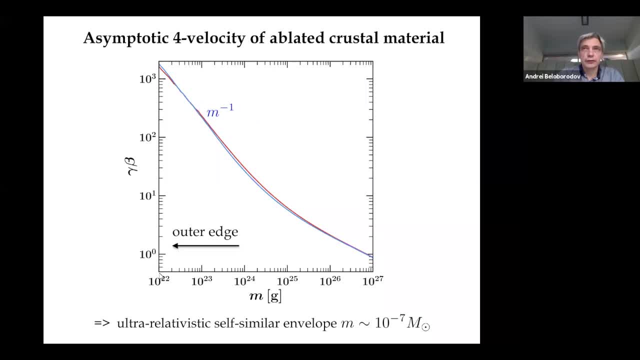 喔, from this region to the outer edge. So m little m is equal to 0 for the first, like the first, like leading front of this ablating material. And as you go deeper, the Lorentz factor of this material decrease. 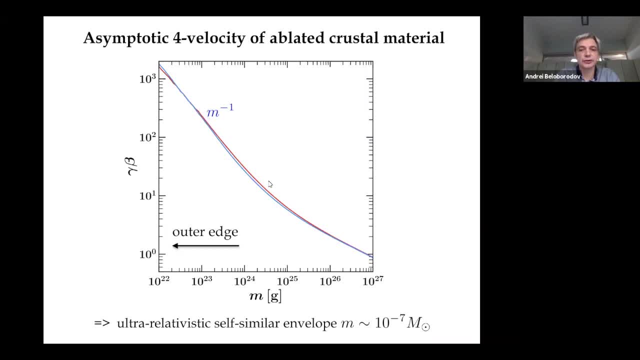 So you can see this huge gamma beta, starting from like thousand, and it goes. you know, there's, like self similar distribution of it. So what you create is a homologous envelope, ultralogistic envelope, ablated by neutrinos with total mass about 10 to minus seven solomons. 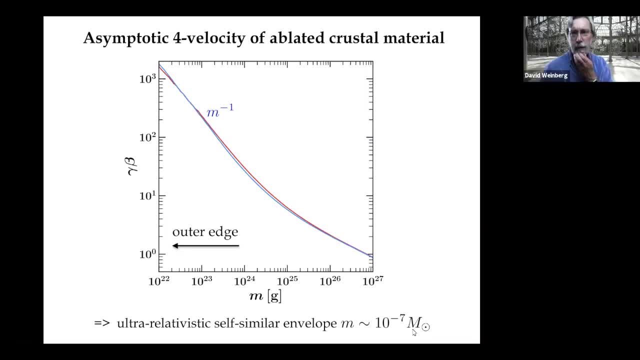 Beta here is just V over C. I'm sorry, Is beta just V over C? So- Yes, beta, oh sorry, Gamma is Lorentz factor associated with it, So gamma beta is full velocity. yeah, Andrei, what sets this temperature of 20 MeV? 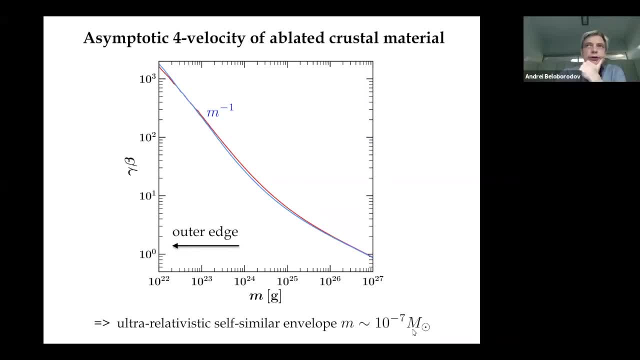 Is it just a real temperature for the shock you said? You know the collision velocity is up to 0.3 C depending on the mass of how compact the neutron stars are. So they have tangential component, they have normal component, but anyway. 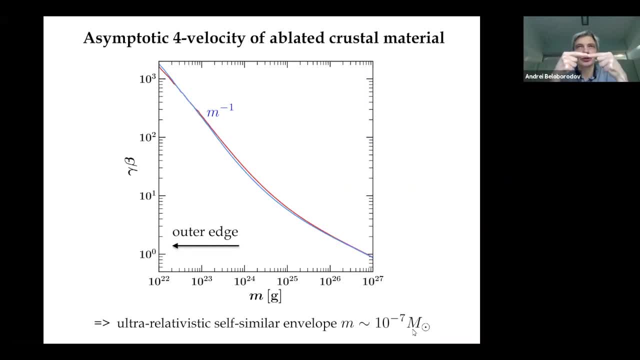 so you know how much energy is dissipated in this collision, per barrier, per nucleon, because you know the relative velocity of collision And this energy, basically, is thermalized in first approximation And that's how we find the temperature. So you know the energy density. you equate it: 80 to the fourth. 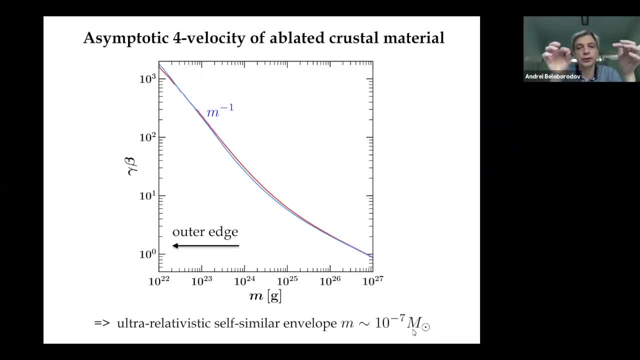 you get the temperature Or, if you like, you just calculate energy per barrier. There are multiple ways of calculating it: relatively efficient, relatively inefficient regimes. In all cases, you find temperature between 15 and 20.. Okay, Andrei, I have two questions, if I may. 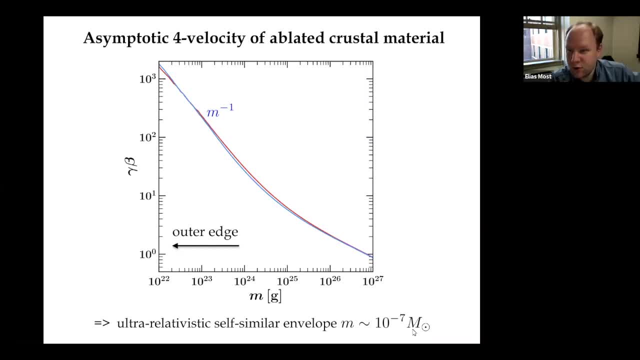 First one is, I mean, is a 10 to the minus seven. what you would need, I mean, this would only come basically from the interface where the two stars would touch. So this would be the order that you need for, like the other numbers, to fit. 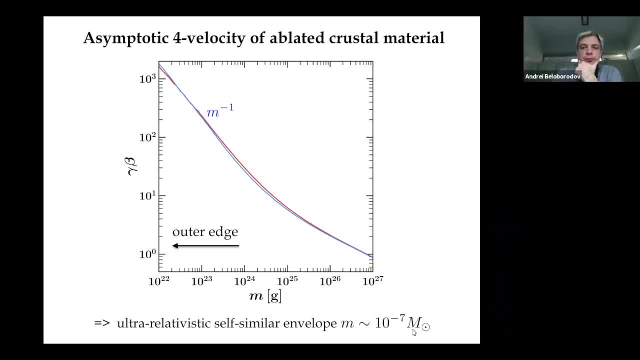 Or do you need more? or What I need for the gamma reversed Exactly? Yes, this is the kind of number, but I will come back to this- The number of the envelope. so this is kind of first principle physics, if you like. 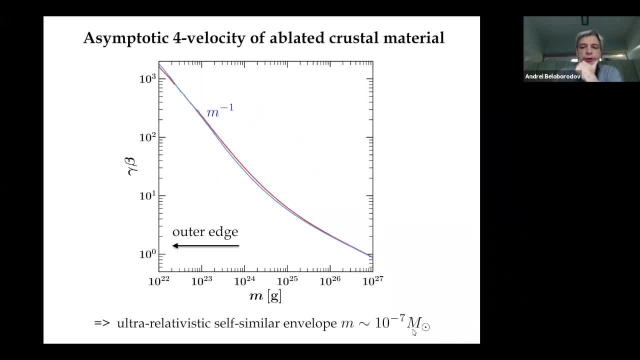 I mean, it's still approximate, but I think that's what you should expect into the minus seven, And I'll look at it in a second. But okay, since you're asking this now, basically, yes, This amount of material is very small. 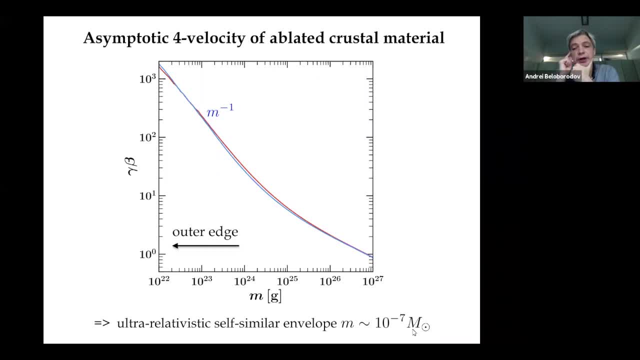 You cannot resolve it in existing numerical simulations. However, when you look at this envelope of 10 to the minus seven solar mass, look at its optical depth: huge And so as it expands with this speed of light, it's basically hides whatever is happening. 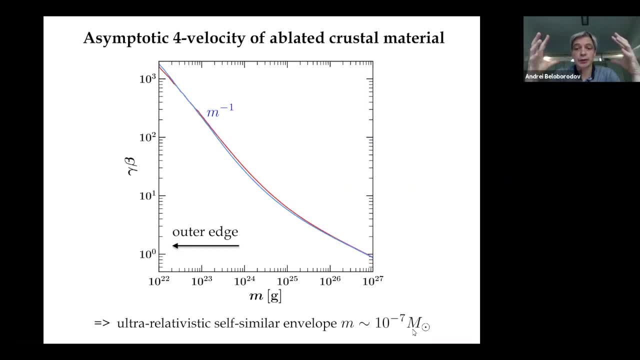 at the center. you don't see because this envelope is fake. It's also cold. the biodiabatic expansion becomes cold, It's dark and not weak And its photosphere is expanding with the speed of light. And you don't see. and it grows. 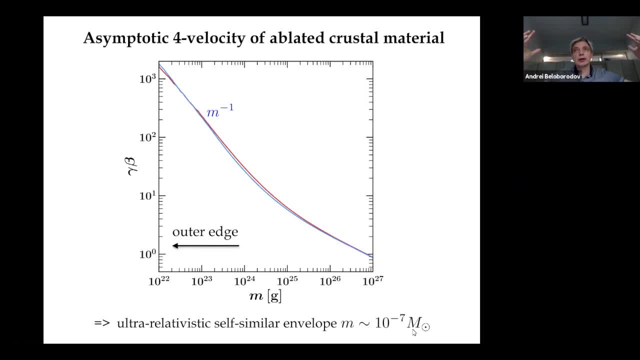 this flow of spectrometers grows with time And you will see later. I will show that the GRB, that which comes from the photosphere of radius, about 10 to the 12th, since the contract, of the larger size, which is like 10 to the sixth centimeters. 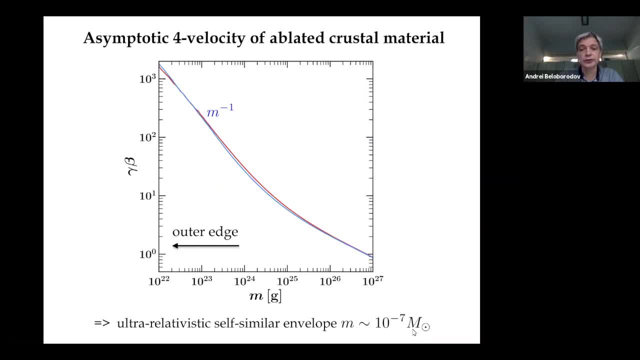 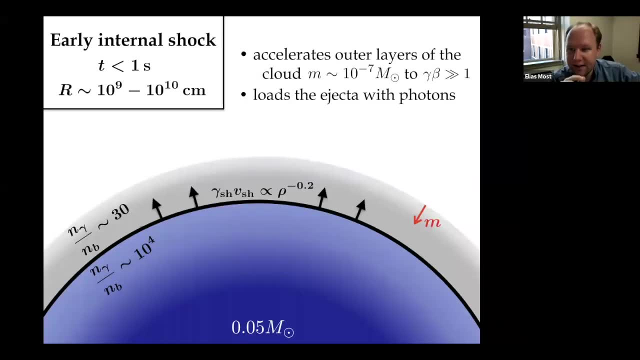 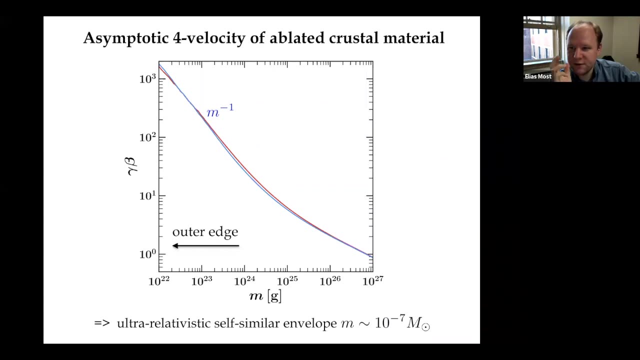 It's million times bigger. So basically the effect of this very light, the dark candle, is to inflate the photosphere of the merger. The second question I had was maybe a quicker one, because you were saying this depends also, I mean, on the collision speed of the two stars. 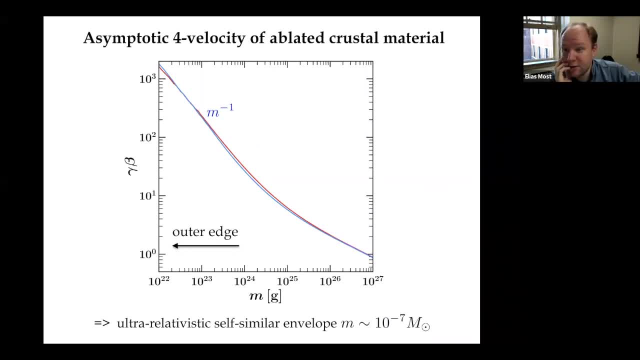 What would happen if, say, I have a very unequal mass merger where basically, you have more tidal disruption going on and less of the central collision? would those numbers like still match or would they go down? Yeah, yeah. So if you have low mass stars, 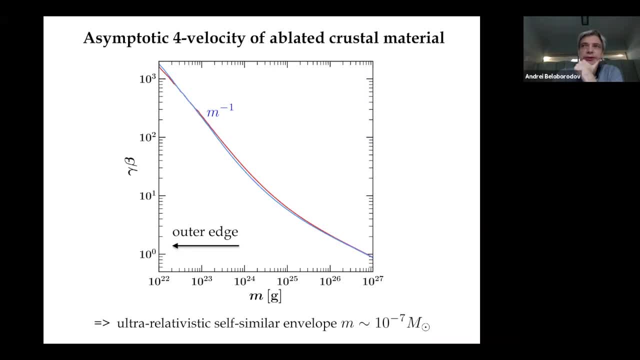 they will go down Unequal stars. I didn't think much about that, But you're right. It is sensitive to the masses of Newton stars. The more compact they are, that is, the more massive they are, the bigger is the relative velocity of collision, right? 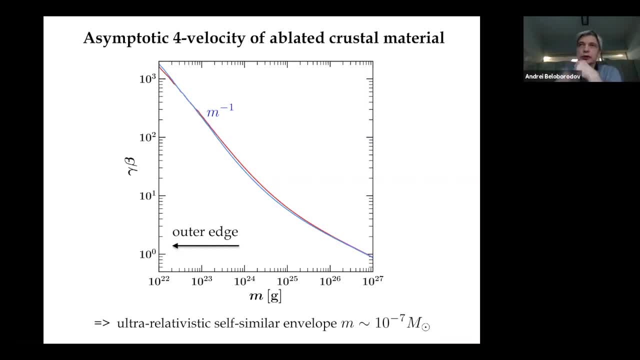 Because they collide kind of deeper in the gravitational potential And you release more energy, more neutrinos, the ablation is stronger, Yeah Yeah. So this is like characteristic number. I took the default like the fiducial model of people who simulated. 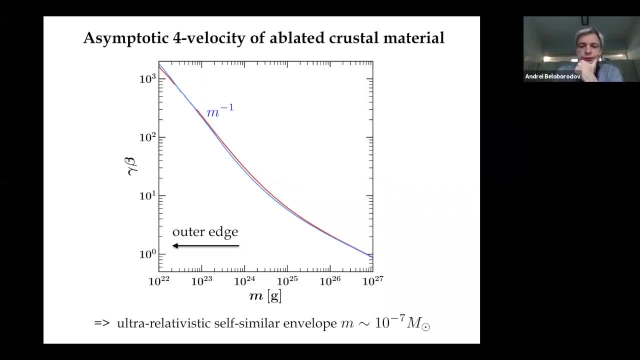 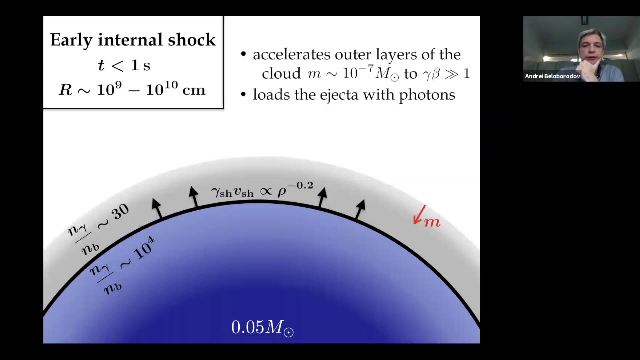 Newton's star with mass 1.44. It could actually be slightly overestimated. It depends on the geometry, because here it is estimated like the isotropic feature, but of course this thing is not isotropic. Okay, But actually I like more that this other way. 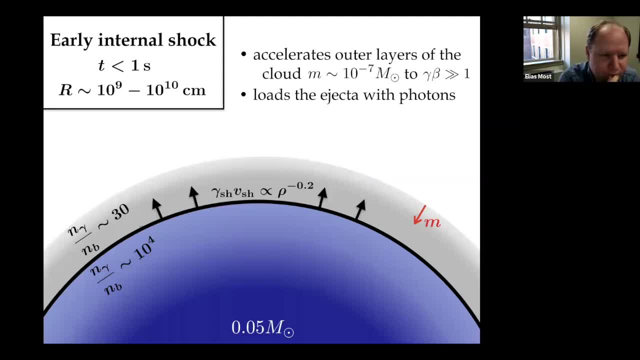 of inflating this envelope, which is robust and simple and also gives itself similar, homologous envelope, promptly, immediately after the merger. If, following the merger of two Newton stars, you launch a shock into this massive cloud, That's the shock that we talked about before. 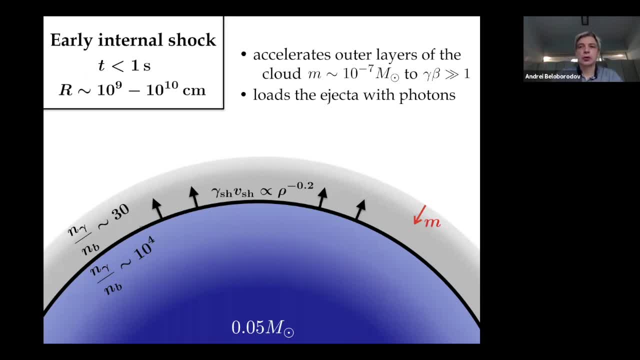 But now I think this shock that happens early, if you actually do the calculation, whatever internal shock crossing the cloud within the first second after the merger doesn't do much in terms of observation, which is the surface of the cloud. photo sphere of the cloud. 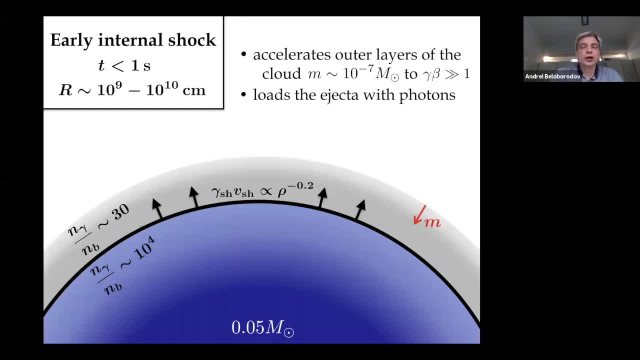 when it has radius about 10 to the 10 centimeters. It has some black body temperature which is slow when you calculate the luminosity from this cloud. because of its small surface area, small radius, it's not a detectable source. 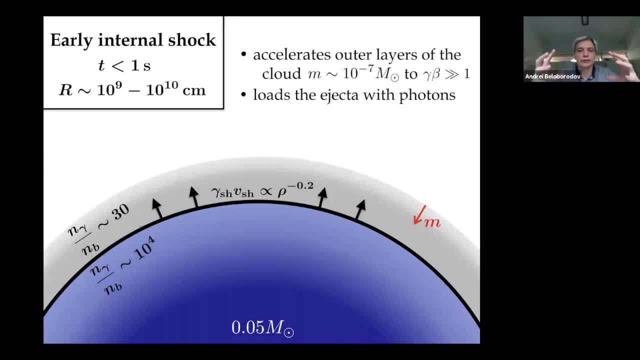 So any early shock that crosses the cloud around the merger doesn't produce a journey because it's too weak. It produces something but it's not observable. On the other hand, it does two important things to that cloud. As the shock comes to this edge, it kicks the edge. 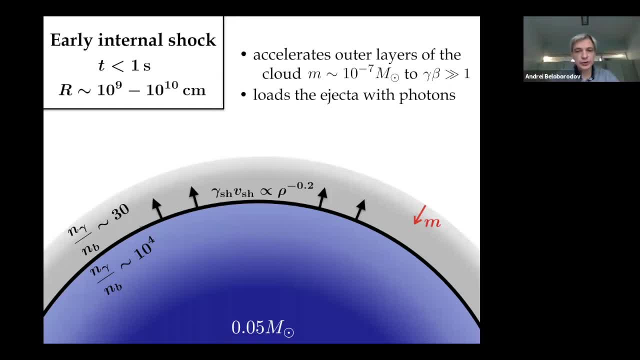 It does this usual breakout business when it pushes the outer layers of the cloud to higher speeds And in this way it inflates an envelope With the extended profile of gamma-beta for velocity of the same quality with the same structure. that is, the leading edge is the fastest. 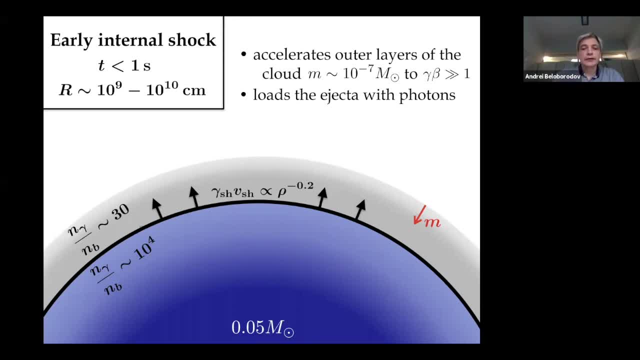 and the trailing layers are slower. So that's one thing, And the other thing is that this shock loads the envelope, loads the ejected material with a large number of photons per barrier, about 10 to the four, simply because it heats the material. 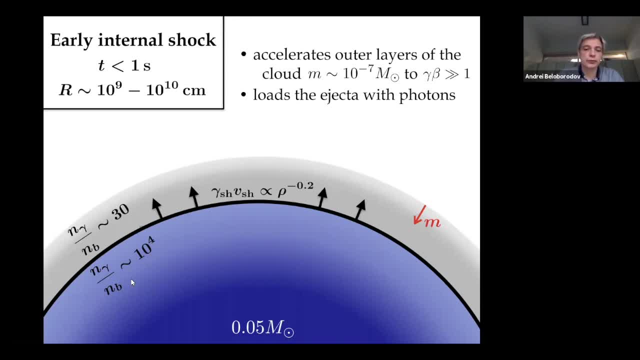 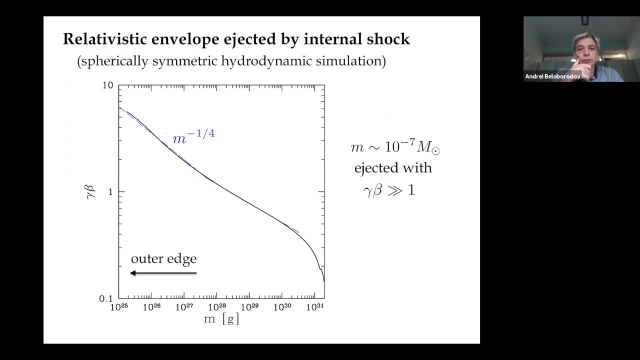 And when you do the calculation you find that it projects about 10 to the four photons Right. This is the hydrodynamic simulation of the early shock breakout And you can see how it is distributed to the mass. So again, little m is mass measured. 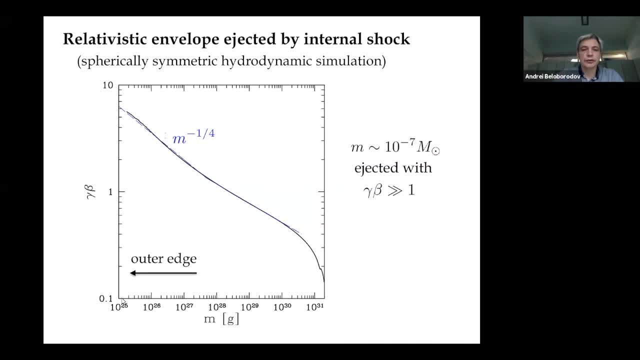 from the outer edge of the envelope, And so the fastest material is at m, equal to zero at the outer edge. And then the scale here is m to the one, approximately. just feed it the numerical results: m to the minus one, Minus one quarter. 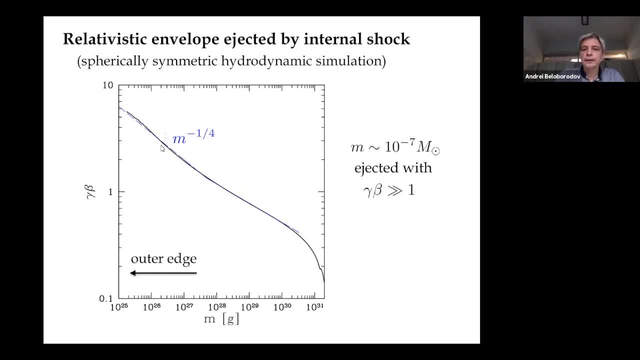 You see it fits pretty well, Okay. And the total mass? in this case it's certainly 10 to the minus seven. Even for gamma-beta-significant, it's a little more efficient and more robust mechanism for producing the signal, So I like this one. 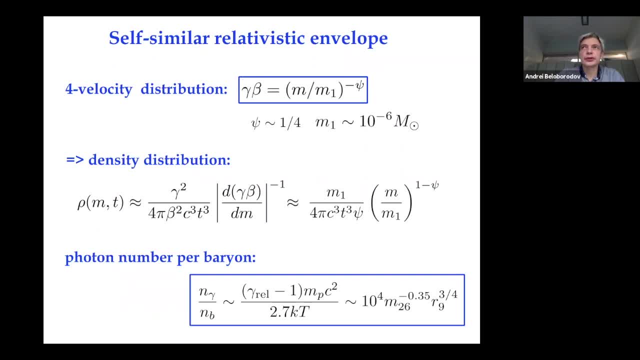 To summarize, I think it's actually one should expect- not only you need it for observations, as I've learned, but one should expect- inflation of the homologous ultra-volatilistic, dark, very light envelope around the merger variant promptly, before anything else happens. 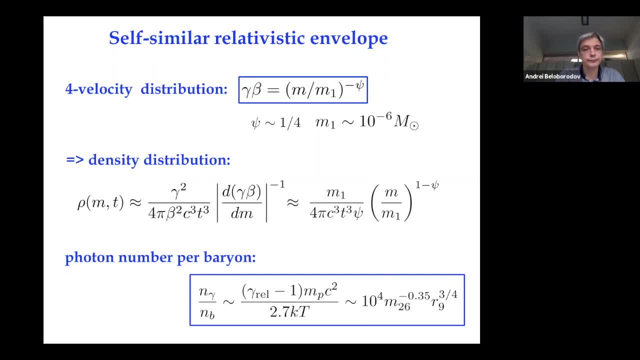 Before the GRB that we saw is immediate And of course you can calculate the density profile of that envelope, which is homologous leaks Like impulsive projection of mass with no loss to distribution. you find it's then density profile how it evolves with time. 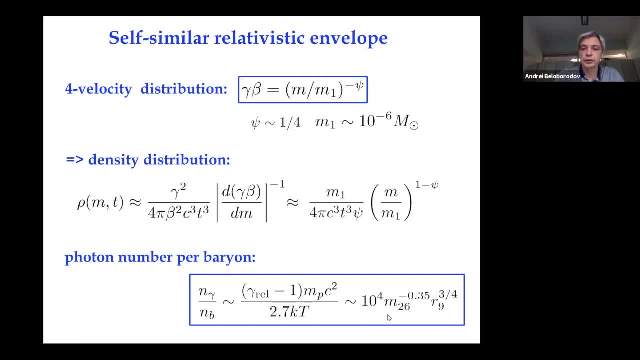 So similar And you'll find the in this lower box. you can see a photo to barrier ratio which is about 10 to the four. Little m here is normalized to 26 grams. That's because we don't see. it's where the photosphere. 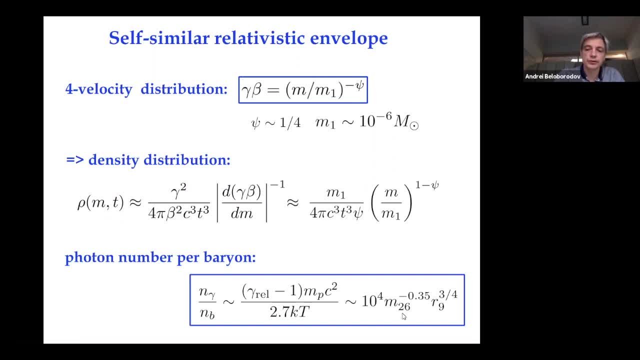 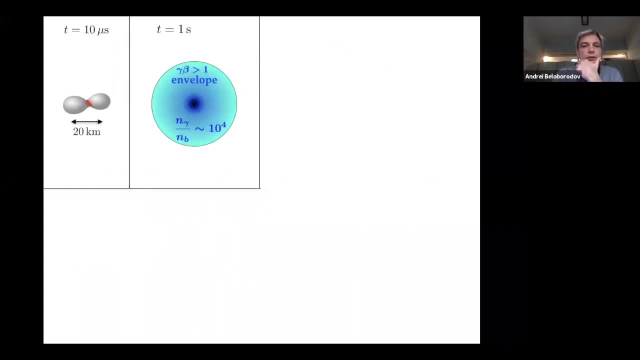 of that exposure. This is the most interesting part of the envelope. This is the part that you actually observe when you look at it from outside. All right, So to summarize what's going on, here, you have Newton star merger at 10 microseconds. 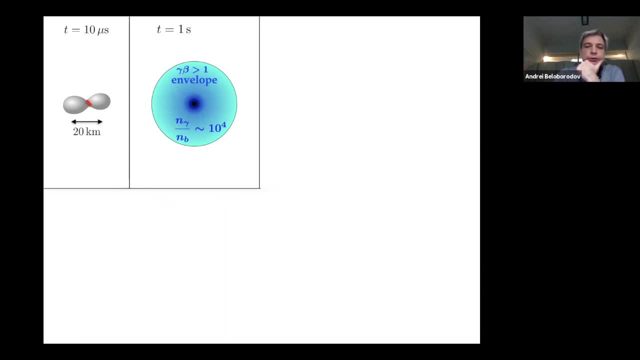 It does ablation, Then you have probably this internal shock especially. I don't want to go into details, but it might be. if you have questions about that, it's interesting to discuss at some point. How do Newton stars merge? 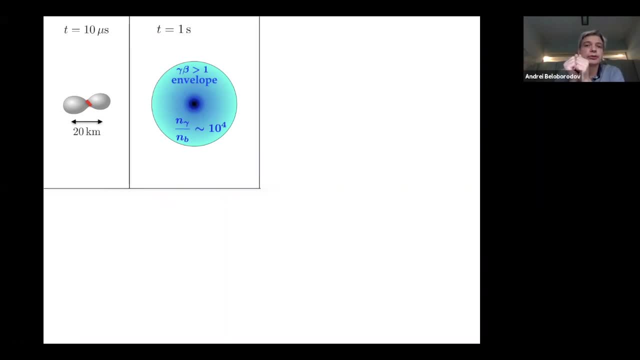 How. we don't know whether the merger product is a massive Newton star. it immediately becomes a black hole. But most likely when a plausible scenario when the Newton star is merged, they lost for a while because of rotation in the supermassive Newton star configuration. Then with some delay, they collapse. The remnant collapses into a black hole, which means that the object, the mass, shrinks. whatever magnetic fields it has in it also aren't too fine, And also you have no clean magnetic field lines because they go into the horizon of the black hole. 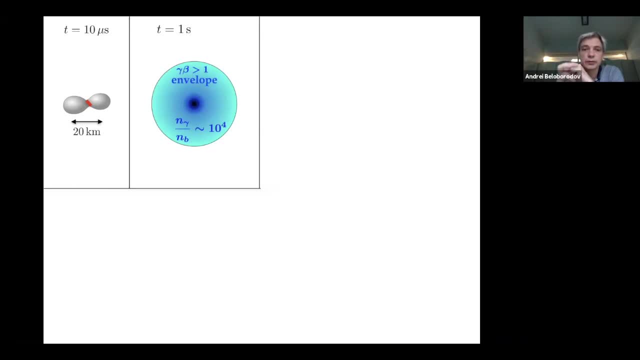 and then you can launch the jet from the rotating, speeding black hole for the. So at that point you expect jet formation with some delay. And so when people argue that, okay, probably why we saw the GRB with the delays, because it took some time for the jet to form- 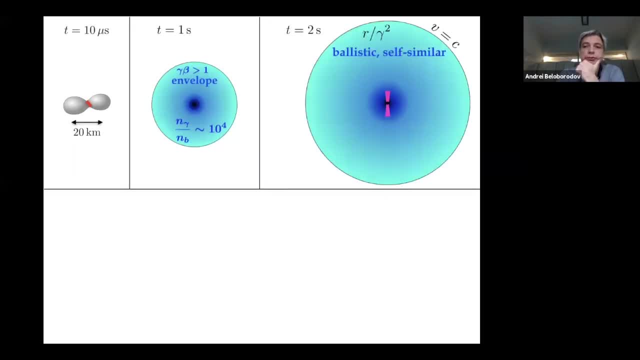 and it could be because it took some times for the neutron stars to form a black hole. Andrei, before you move on, I just wanted to clarify one thing. So this merger and this expansion of the bladed material takes place in a vacuum, right? 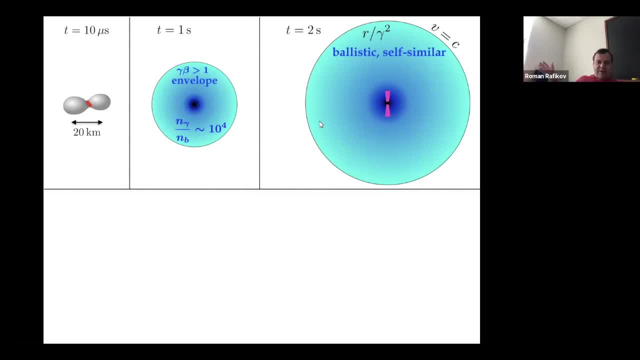 There is no like wind or anything that happened before, From the binary before anything happened to the black hole before they touch. Yeah, So this ejector, this ablated ejector, just expands freely in vacuum. Yes, that's the picture, But of course, in reality, if you put an obstacle to it. 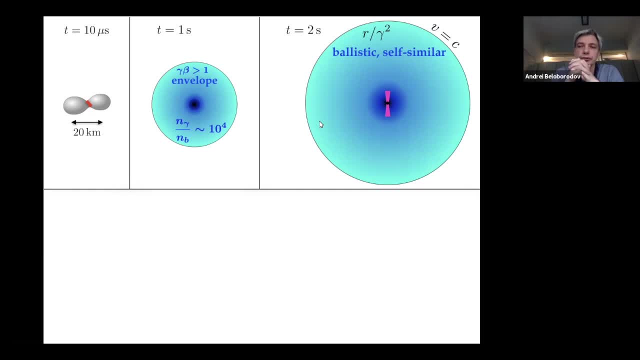 then you have to think about how this- the wind- compares in density and Lorentz factor with your-. Yeah, but there is no obstacle, right? I mean you're saying it's expanding in a vacuum, because I mean you started by saying that. 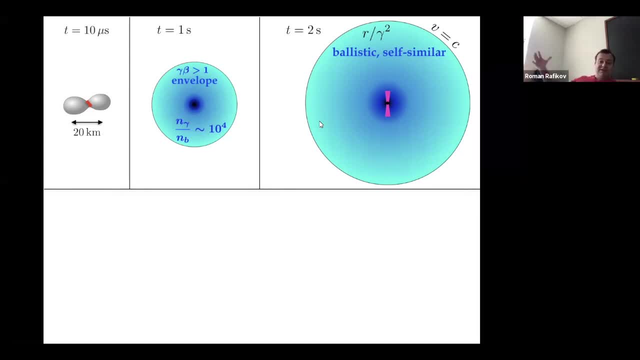 it was a short breakout from something, So as if there was some kind of preexisting envelope already. So- Okay, Okay, So that's yeah. So not to confuse. So the picture is like this: You have two neutron stars. they merge. 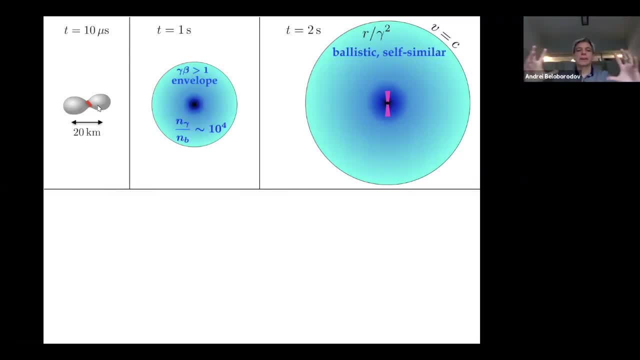 Initially, let's say they're walking around nothing. Yeah, They ablate some material. okay, ultra-OTBC, very little mass. It is followed on a timescale of seconds. Also, it's shown by hermeneutical simulations. 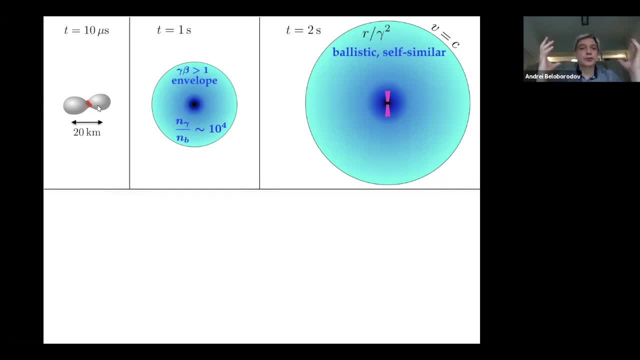 By ejection of a lot of mass, like percent of solar mass, 5% of solar mass. that we will observe later as Q1O. Okay, So this material is moderately typistic, expanding with speed about 10 to the 10th centimeters. 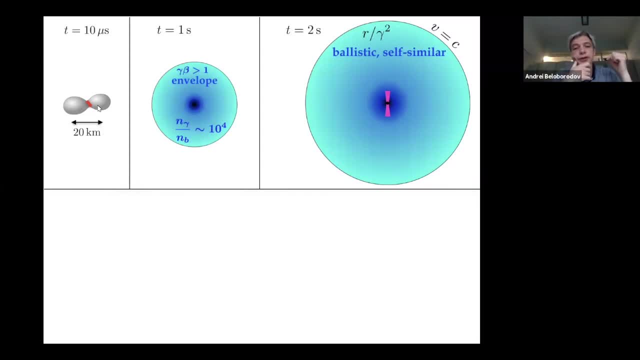 per second if you cancel the speed of light, If at the early stages, after you form the cloud, it is crossed by an internal shock from the merger. For example, you had the magnitude wind because this supermassive still alive neutron star. 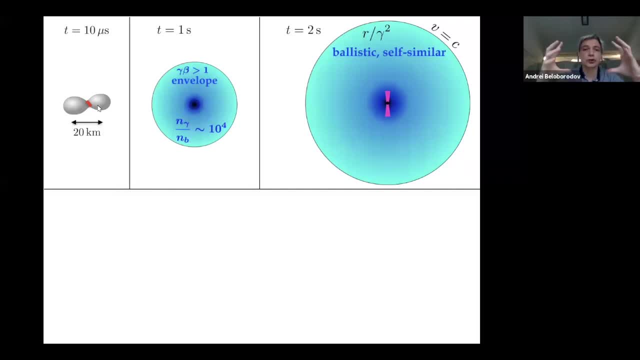 would act as a magneto launching magnetized wind. maybe drove a shock, Or maybe there was just a shock coming from the meter itself. If a shock crosses this early still, small in size, massive cloud, as the shock comes to the surface of the cloud. 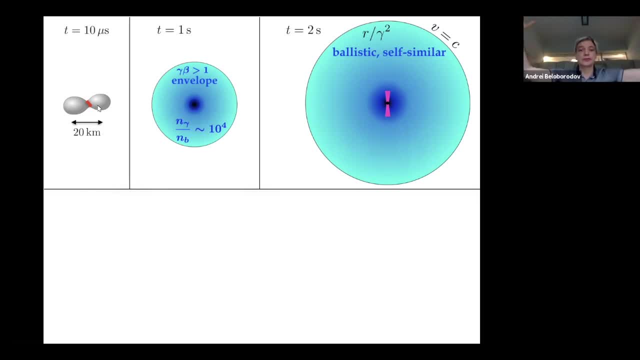 it kicks its layers and inflates immediately ultra-Oletabistic envelope around. Okay, so you create the structure roughly- this is what's pictured here- t equal to one second. you generate- you expect to generate- a massive cloud. it's the kilonova, the dark blue. 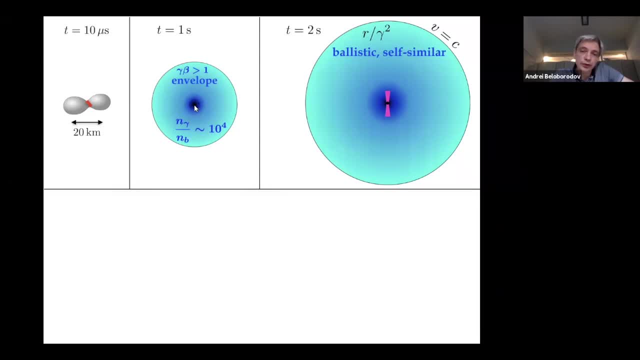 it will. this is future kilonova stuff: dense material, ultra-rich radioactive Around it. you have inflated this ultra-littlistic envelope. at the edge of this envelope, full velocity diverges, okay. so when you do the calculation, 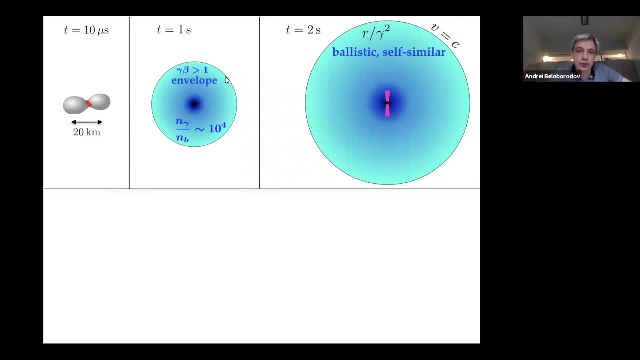 if you forget about the positives. suppose it's completely epic. it just diverges. So you have a horizon. it's like when the jet is finally launched from the center. it expands now not in the vacuum, not an external medium, it expands in a new universe. 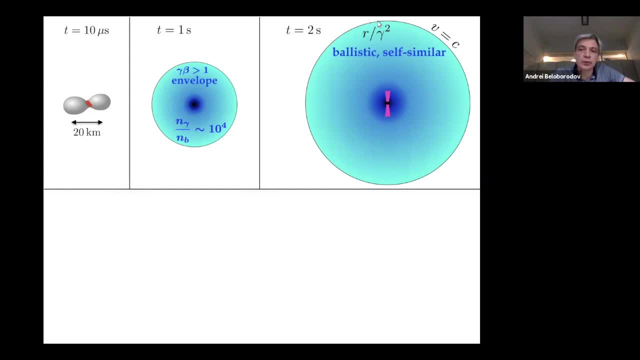 which has unreachable horizon, running away with the speed of light, and the jet is ultra-littlistic and of course it will catch up first these deeper layers which move slower, with lower gamma and as the time compresses. 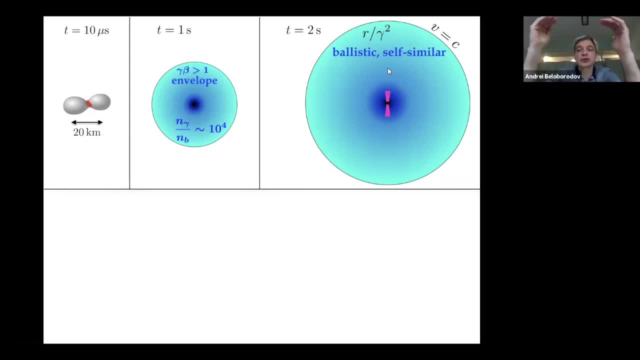 the jet will keep catching up fast and faster layers, but it has no chance, of course, to reach the first layer, which goes along with the gravitational waves. they go with the exact speed of light. let's say That's the basic picture. 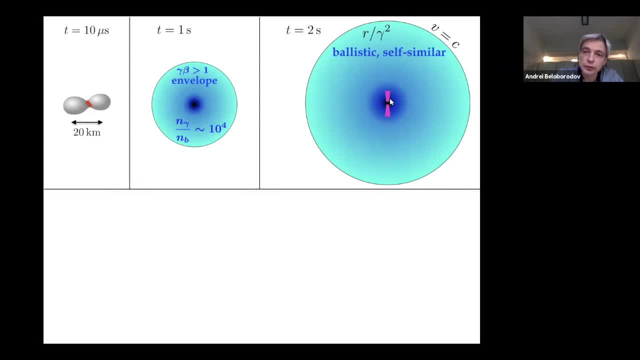 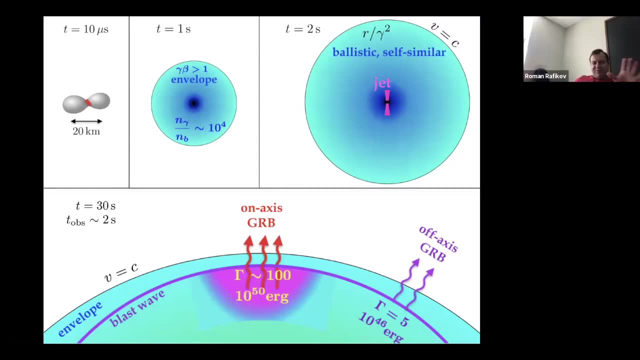 and then here behind this, you have this dark blue which is the future kilonova. Okay so light blue is your ablated stuff. dark blue here is the kilonova stuff, Ben's stuff. yeah So dark blue is 5% of solar mass. 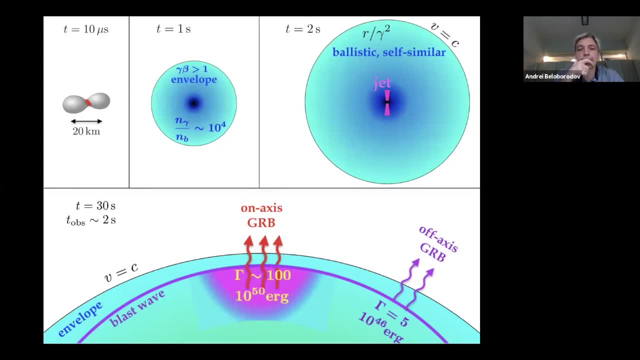 and light blue is 10 to the minus seven solar mass. Okay, Thanks. And so this envelope is going to be very neutron-poor, right, because it's coming from the neutron star crust. I mean, that's not going to-. 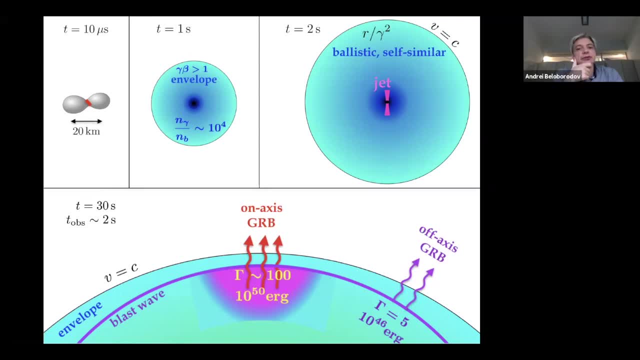 It's a good question. It's yeah, there is nucleus synthesis. It's not radioactive material. It says it's not very efficient for our process. I think I'm not sure how rich it is in terms of. so it does come from neutron stars. 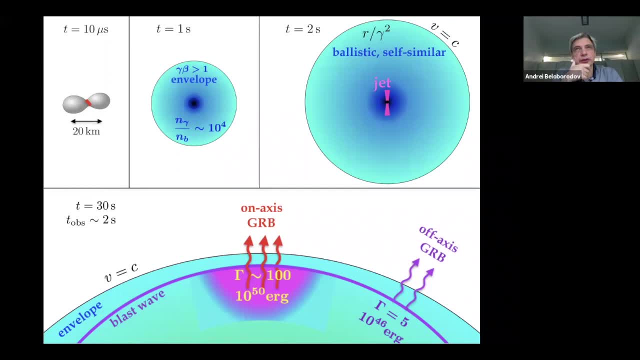 but the YE, the ratio of protons to barriers, is regulated by neutrino emission and absorption, And so it is changed from what it was originally. so, of course also, it's completely decomposed at high temperatures into free nucleates. Then, as the stuff expands and cools down, 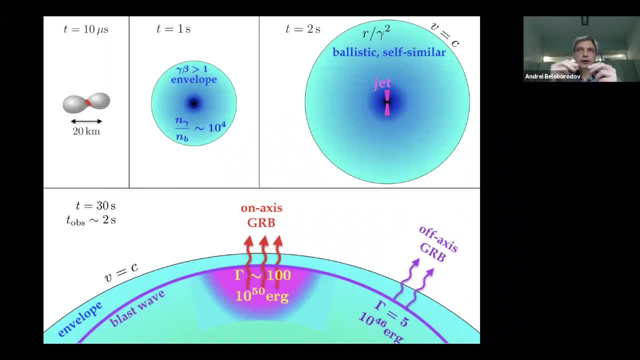 the nucleates tend to recombine into kilone. and then there are some also some leftover nutrients. So there are more nutrients than protons, but it's not really clear by how much. But you're right, There should be some nutrients also there. 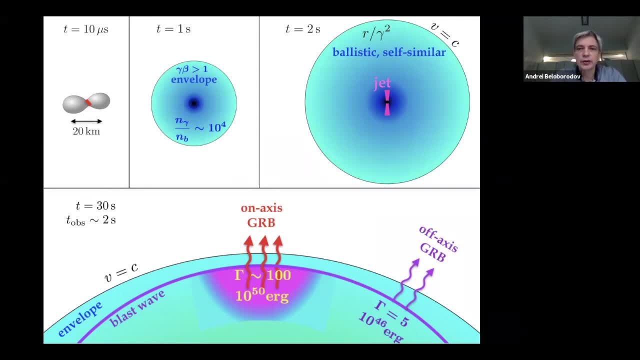 There's a nutrient component which actually is an elephant in the room, if you think of it. I wrote a few papers about this some years ago. All in the entire, GRB theories construct as if there's no three different component in the GEN. you know the canonical GRB models. 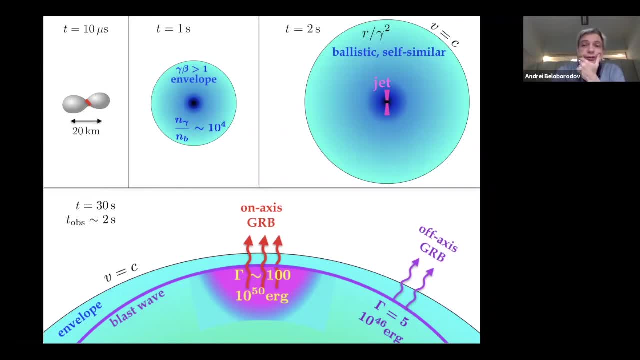 But in fact there aren't three neutrons and they do affect stuff, But it doesn't affect the. I mean, you still have the envelope, you still have the kilovolt cloud, you still have the GEN, You still the jet still has to drive a blast wave. 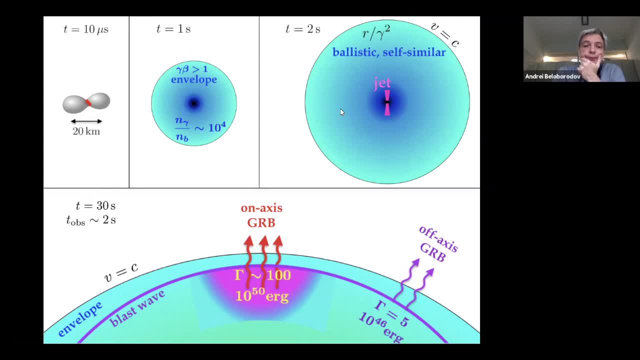 into the envelope. So when the jet comes to the photosphere it will radiate gamma-ray burst And you can calculate. let's say, if you meet 10 to the 46th, if the energy of the blast wave 10 to the 46th. 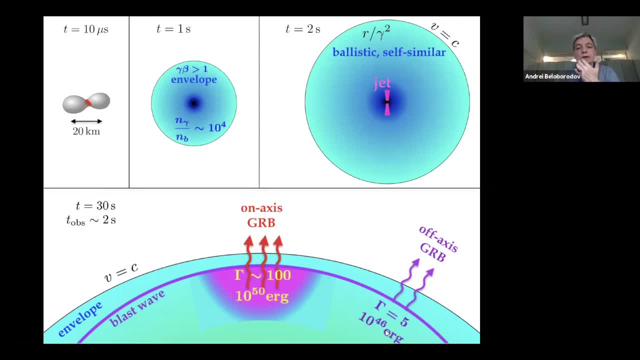 and to the 47th arc as a tropic equivalent. Of course it's much higher on the axis because the jet is, you know, collimated, So the blast wave that is launched by this jet, so it will drive a blast wave into the envelope. 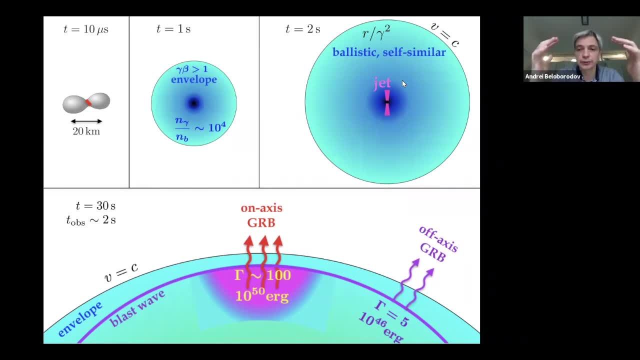 It will not have as a tropic power, because the jet is collimated And how it is distributed over angle we don't know. Actually we're working 2D simulation but I don't have an answer yet, Assuming that at 20 degrees. 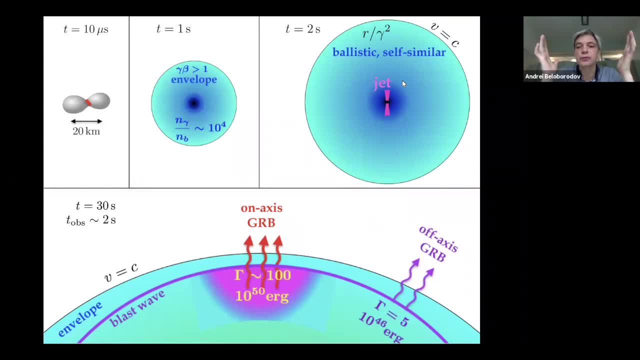 it has power which is like three quarters of magnitude lower than on the axis, which seems plausible And it seems like, well, it's not finished, but hopefully it works out. this way, You do produce GRB with the right properties. 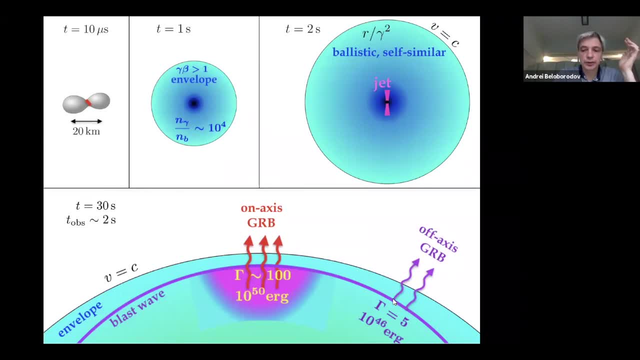 And that's the main message of my talk. I will try to explain now how you generate the gamma rays that you see by this blast wave. So the main point is that after you inflated this envelope and launched the jet with drills through the massive cloud, 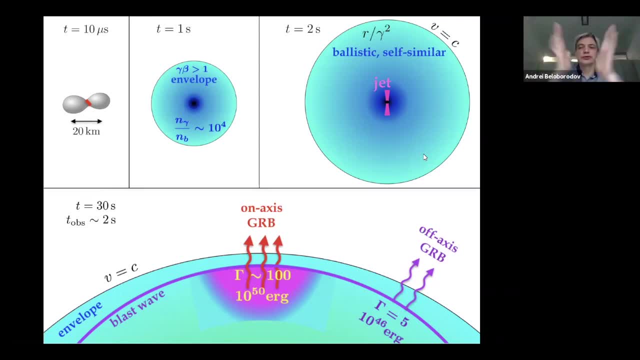 and then it goes into the envelope with jet break up, it launches a blast wave that eventually is not seen because the envelope is opaque, But eventually this blast wave has to come to the photosphere and radiate, And the spectrum of that emission is a gamma ray spectrum. 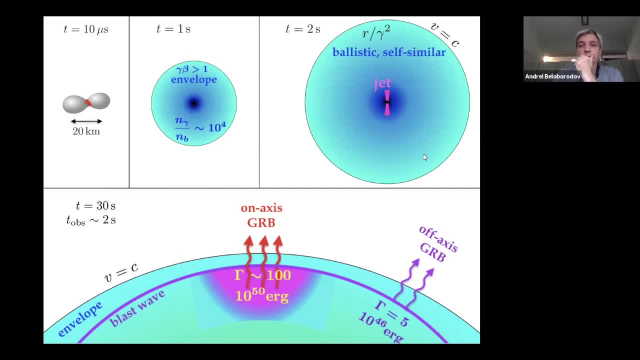 that we observe. I think One can also quickly estimate it. So that's why it picks up. It picks up a hundred KB. but let me just move on now, because I think I'm a little- yeah, I'm a little slow. 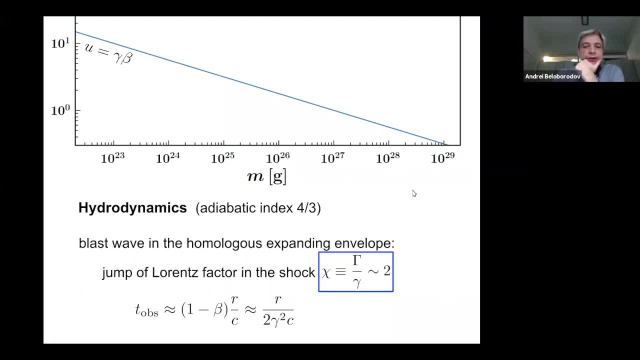 So let me just explain, Let me show. first have an image, simulation. So gamma beta, this full velocity profile of the envelope. This is how it scales with this Lagrangian mass coordinate. Again, remember, M is zero at the outer edge. 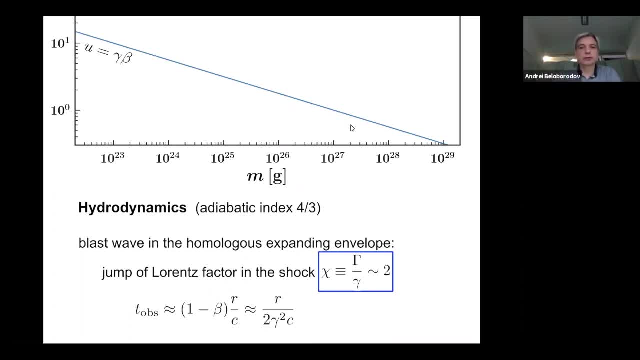 This is stratified density. So if you launch it, this blast wave into this expanding envelope, that's what you will get. so the jump here. So there's the material, which is faster, right, There's the shock. the jump here. 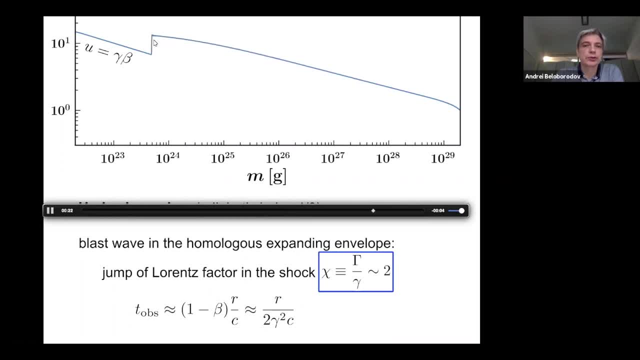 that propagates through the envelope And note that it remains. the jump remains approximately constant, shrinking slowly, Eventually. if you run it into the time it becomes almost nothing, But for many decades, in mass, the jump remains almost the same. 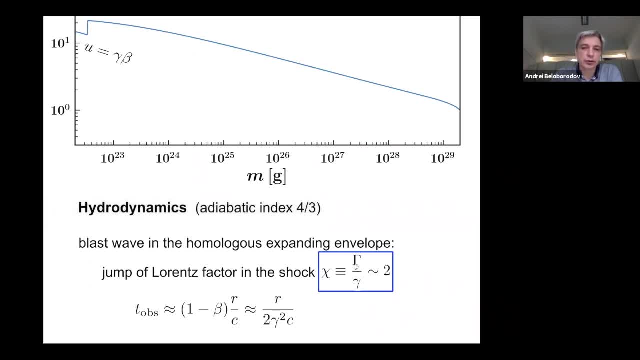 So if you introduce the sky parameter, which is the strength of the shock of the blast wave, it's the ratio of the post-shock downstream gamma to the upstream, It is the jump of the Lorentz factor across the shock. It's about a factor of two. 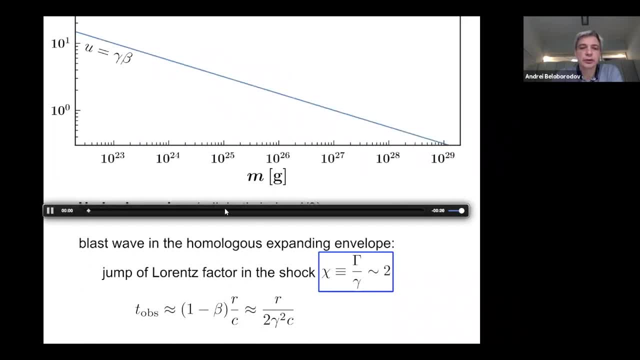 Okay, and it stays about a factor of two. I can run again: It stays about a factor of two to the range of mass The photosphere is about. here it turns out So, even though the material is moving out at essentially the speed of light, 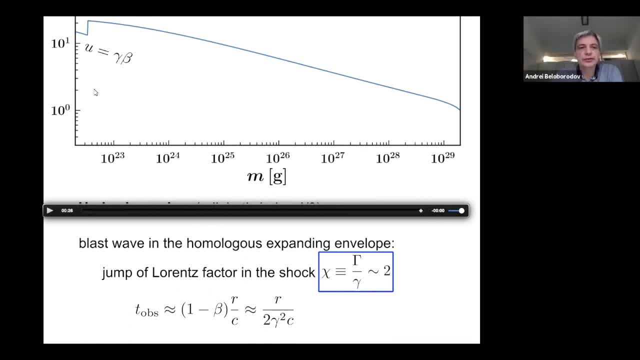 the shock is able to catch up with it. Exactly so the material is. so if you look at the state of the shock, let's say here the shock has caught up with the material, which has Lorentz factor of about three at this point. 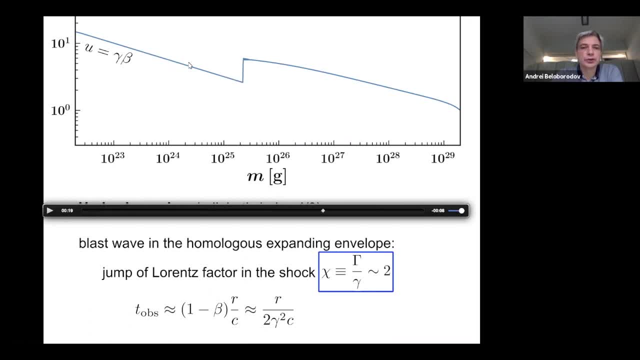 And of course it's still. it has not reached even faster material which is just next to it, looking at Lagrangian chord. It will have to wait longer to catch up faster material and longer to even faster and longer. 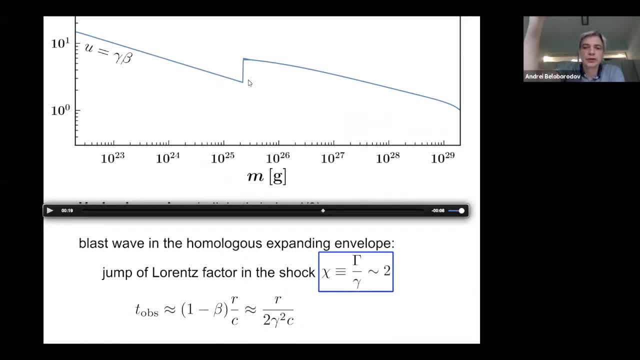 So it's racing toward the outer edge. but even if the shock- and it does move with almost speed of light, the layers ahead of it also move very fast And the time it takes to catch up is roughly is proportional to their relative. 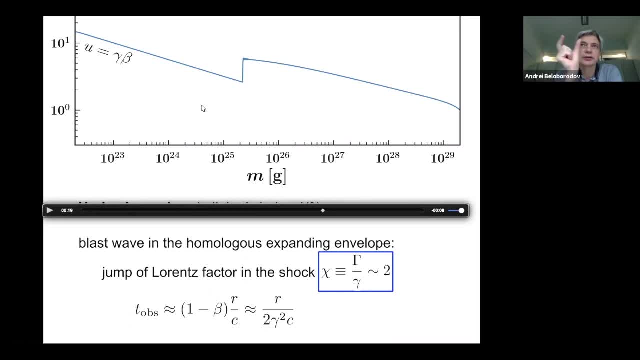 inversely proportional to their relative force, one minus beta, Where beta is the upstream loss to that you're targeted at trying to catch up. The closer beta is to unity, the longer it takes you to catch up with it. Okay, So it's also similar, right. 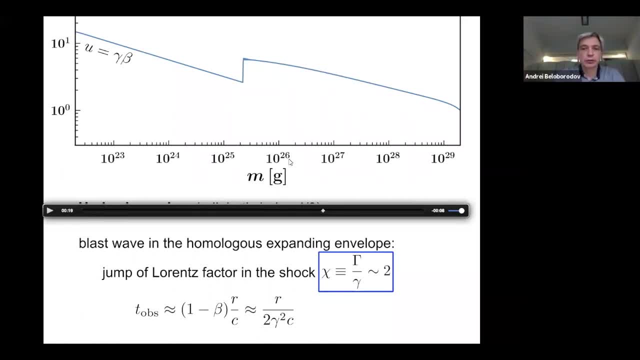 It just you launch a shock wave into this homologous expanding envelope. You know the properties of the envelope within the factor of review, like its profile of gamma beta. you know you have an idea of the energy of the blast wave. 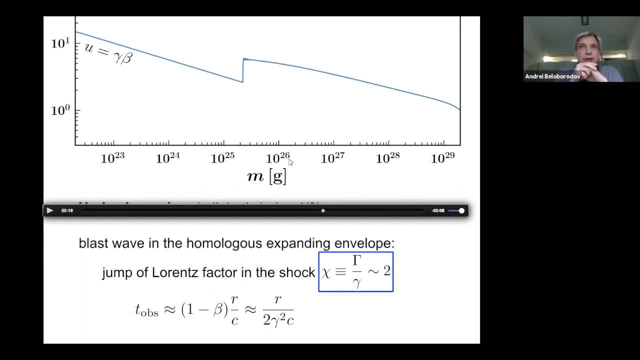 it is in your direction because you see it, And that's it Here at the end of the problem formulation. you want to know the spectrum of the blast wave that emerges from that envelope. You don't have any free parameters, really, in this problem. 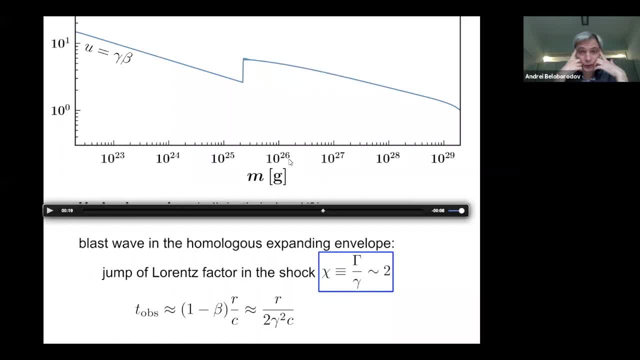 You can calculate from first principles the dynamics of the blast wave from the initial of the blast wave. It's not easy but I will show you. we've done it now And the paper is unpublished yet, but it's submitted just a week ago. 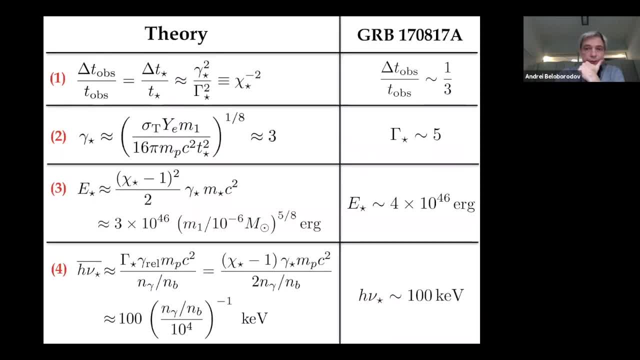 Okay to summarize the theoretical properties, but they should observe properties of this blast wave. It has one funny property that I wanted to highlight: The duration of the photospheric emergence of the blast wave at this photospheric radius r star. Star means photosphere here 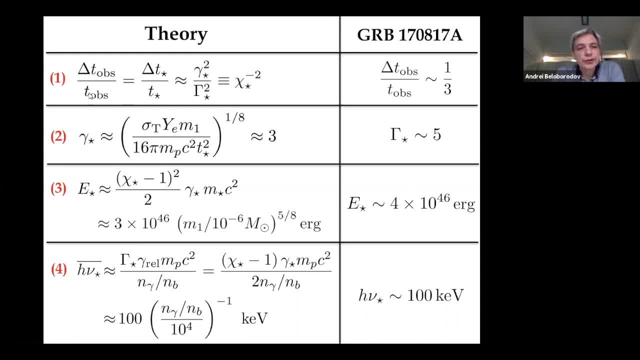 So the delta T over T at the photosphere is basically the ratio of the Lorentz factors upstream and downstream. This is the jump spirit Reason. why is that? because the observed time it's how long it takes for the blast wave to catch up. 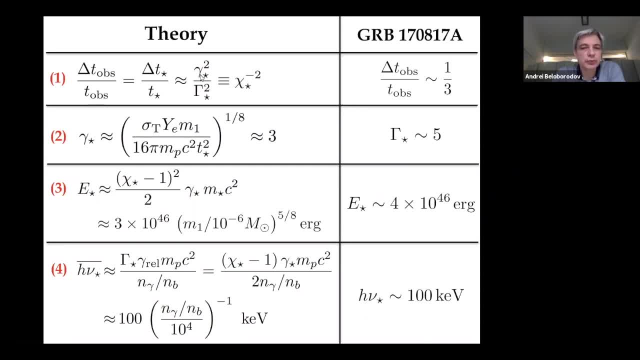 Scales is one over gamma square. This radius, divided by gamma square, divided by c little gamma square. The duration, though, is set by the downstream Lorentz factor. gamma, It's a, it's a hot shell, which which moves faster. 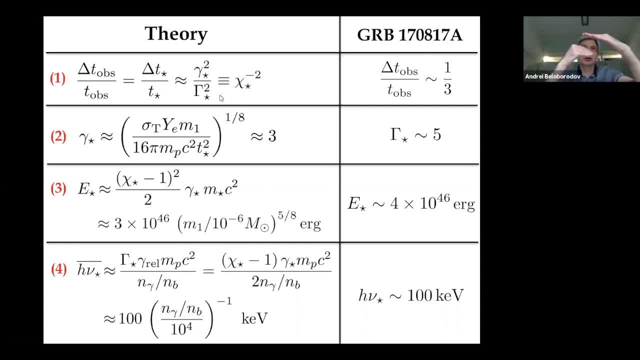 And the duration of this Doppler compression corresponds to its own capital gamma, faster gamma, And so the ratio of delta T over T is just the ratio of the two Lorentz factors. So this model predicts that this ratio is a few and the observed ratio is indeed one third. 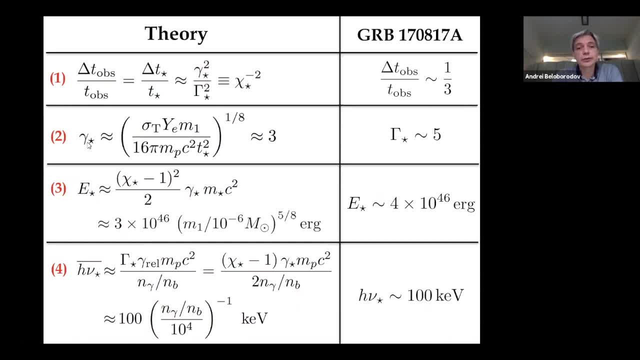 It's quite consistent. Then you can also calculate the Lorentz factor of the envelope layer which will serve as a photosphere, And it's basically three Scales, is one to the eight, And when you apply that chi star ratio, 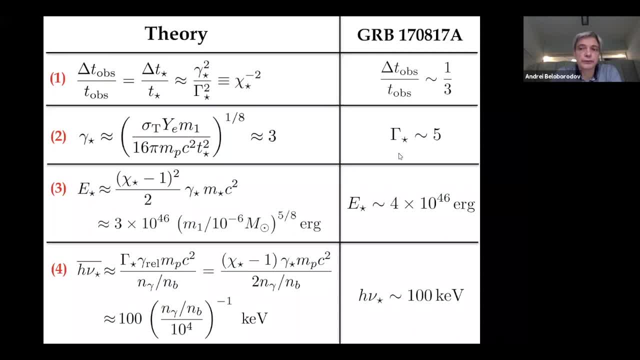 you find the ratio is like square root of three. We find that the capital gamma, the downstream, the source gamma, is five. Remarkable. of course, it's the same five that I told you before. So it's where the two lines, the two constraints. 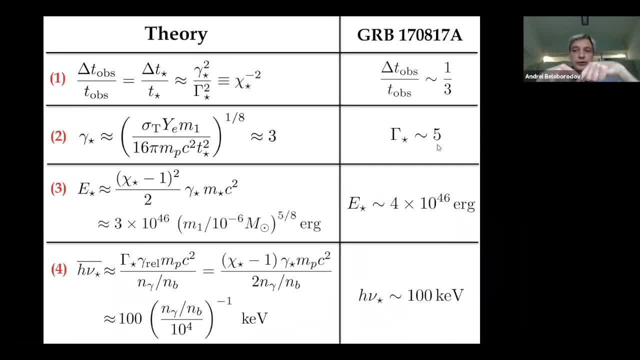 remember I showed the plot with constraint cross. That's exactly what the source should be, because what I'm talking about, the photosphere, the photospheric condition, Its duration lies in one line and its opacity is one. It was the other one. 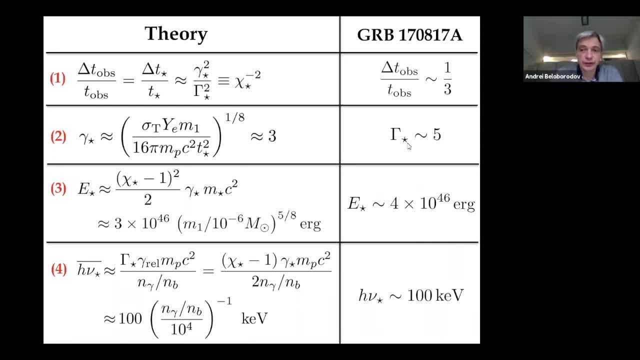 So of course it's where they cross. It's exactly gamma's five and it does work out to five And you can calculate the energy that is produced by this blast wave And you know the strength this natural purity times. you know the Lorentz factor of upstream material. 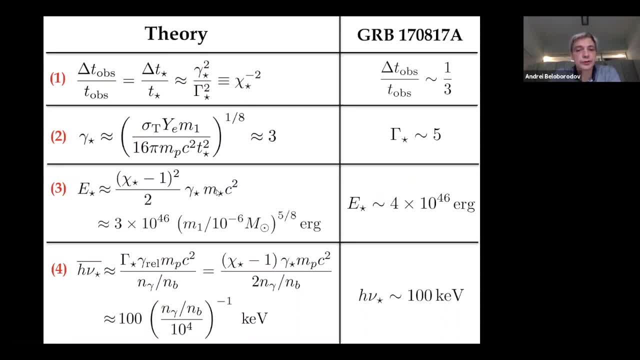 times the mass. And the mass you also know, I told you, is 10 to the 26.. You can calculate it in this envelope And you get a number which is consistent with the observed energy. And, finally, you can calculate the typical characteristic. 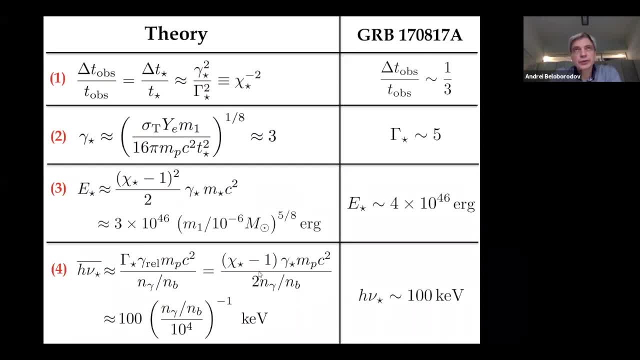 energy of the photons And, not surprising, the blast wave basically hits the existing photons in the envelope And I mentioned before that you can estimate how many photons you expect, And it's 10 to the four photons per barium. It translates to the energy per barium. 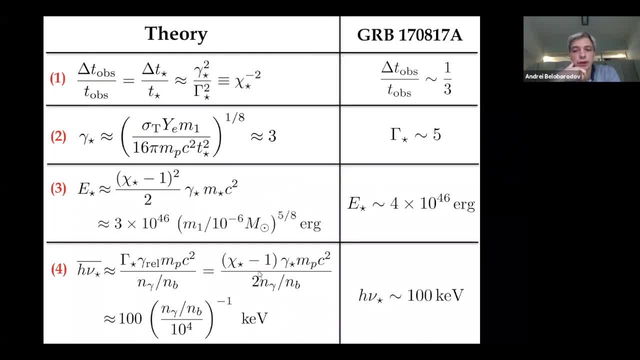 Energy per photon in this photosphere commission about 100 kV, and that's what's observed. So to me it was really convincing. that it's. I was excited about that, And so we with Christoffer Luhmann. 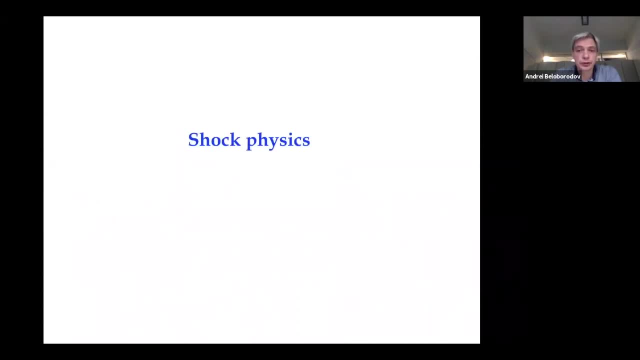 we've done now the full simulation that actually calculates the spectrum. I don't think I have time, So how much time is left for me to talk? Well, we should probably try to leave it five to 10 minutes at the end for questions. 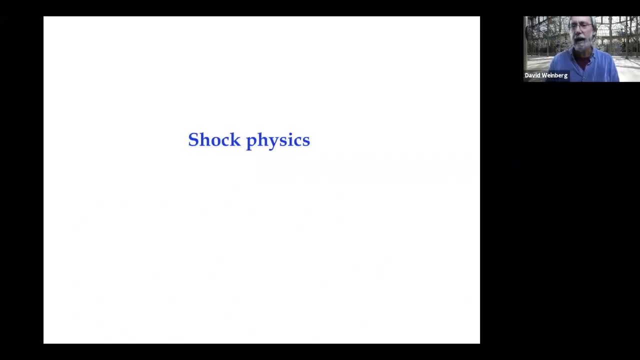 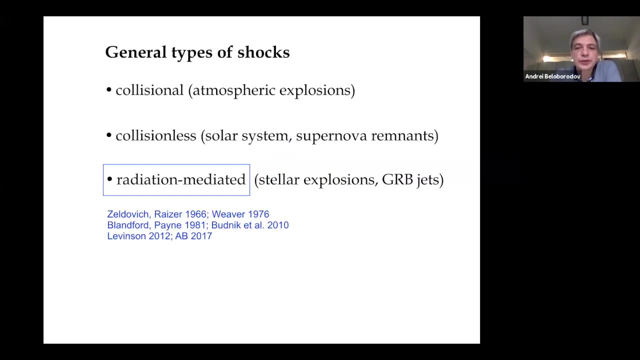 So if you could finish the talk in the next five to 10 minutes, Five to 10 minutes, that's good. So I was planning to talk more about details of shock physics, but I will go quickly and show the results of this first principle simulation. 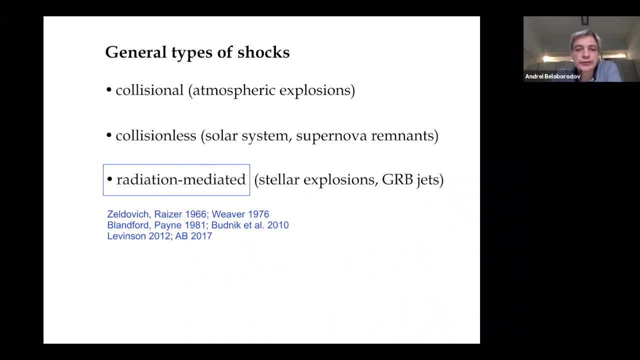 that we have for the shock breakout. So I would like to emphasize that this blast wave is a shock wave which is mediated by radiation. Okay, So there are different types of shocks. There are collisional shocks, like atmospheric explosion, collision-less plasma shock. 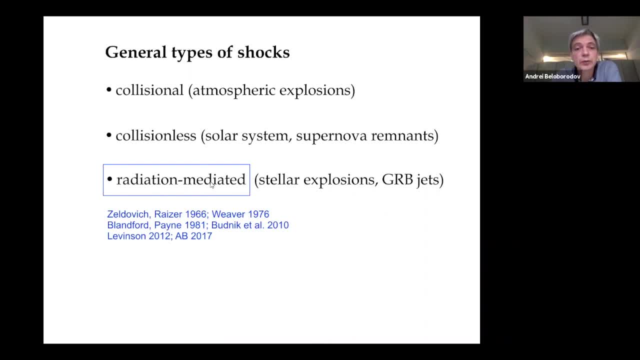 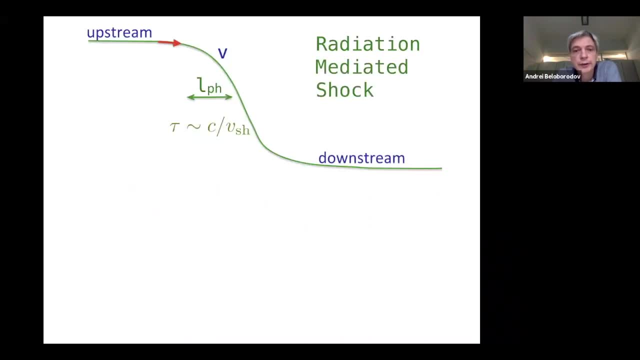 solar system supernovae, for example. Here we're talking about shocks which are originally launched in opaque medium, which is radiation-mediated shock. So this shock works like this: You have upstream, In the downstream, you reprocess the energy into radiation. 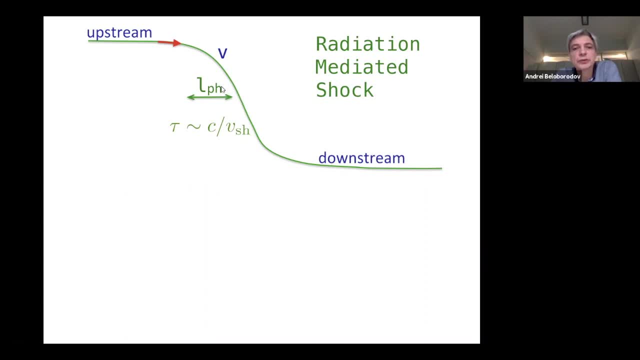 Secure pressure is completely dominated by radiation. So the upstream and the velocity profile and the velocity profile and the velocity profile of that shock is regulated by how radiation pushes back onto the upstream. It's like upstream comes to this radiation and sees it's like a pillow. 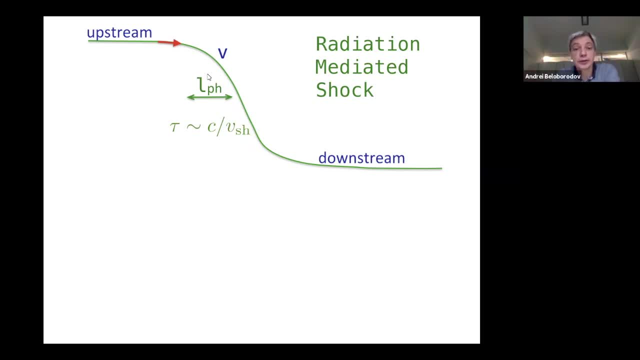 decelerating it smoothly, gradually, by the radiation pressure. So the thickness of this transition and velocity is comparable to the photon-free path for relativistic shocks. The plasma in these shocks, because they're so relatively broad, the photon-free path. 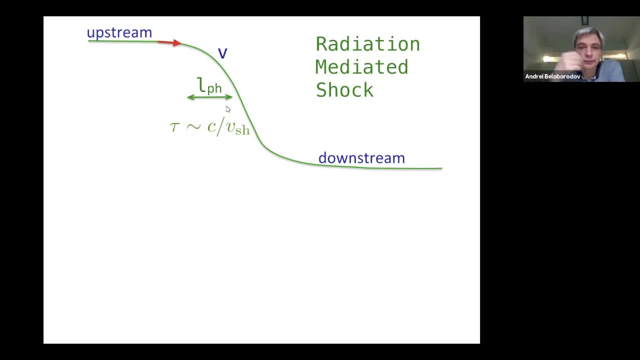 let's say the photosphere is comparable to the size of the system. okay, So it's a really broad transition. The plasma stays completely in equilibrium with the kinetic equilibrium with photons, So it has constant temperature, about 10 kV, everywhere. 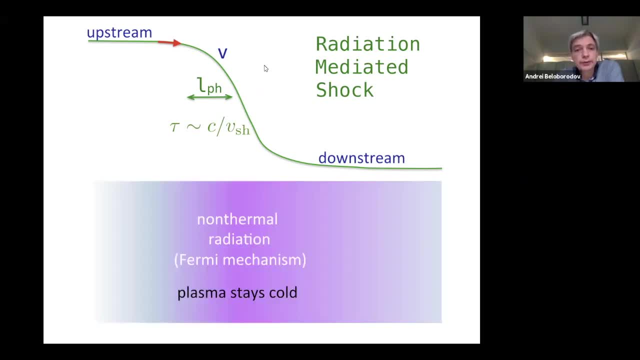 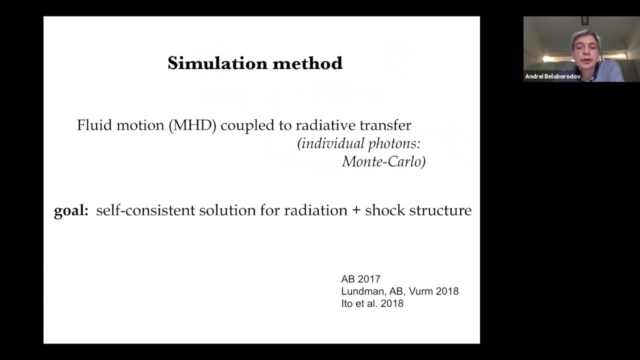 But the photon spectrum in this shock is not thermal, because the photon bounce on this free path between upstream and downstream and, just like the thermal acceleration, it's not thermal. So the plasma stays cold, but the radiation becomes not thermal. We developed a method to simulate it. 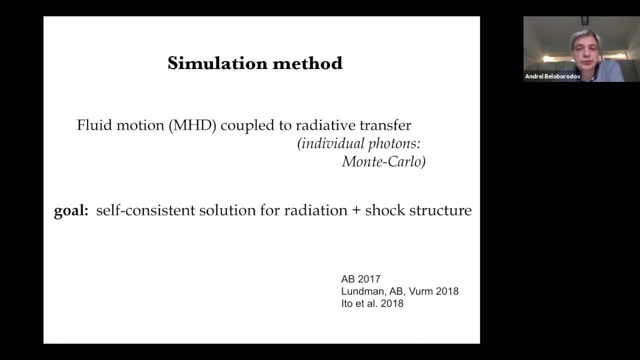 from first principles. Basically, it's MHD coupled to radiative transfer done with Monte Carlo. So we pull individual photons, many of them billions of photons, tens of it's, not billions. I should take it back. 10 millions is enough. yeah. 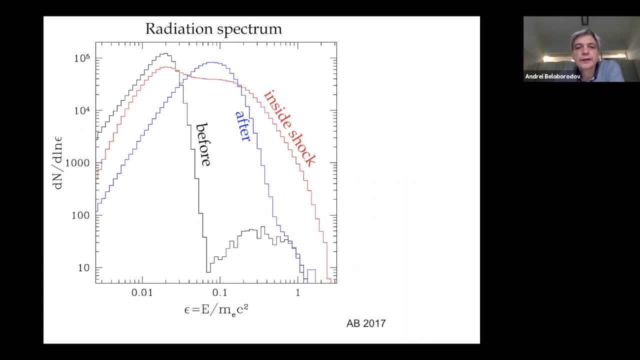 I mean, unless you do simulations, This is the spectrum of radiation before the shock, which are some thermolapse radiation, black line. After the shock, you just heat up the photons. far downstream that's blue, And inside the shock because of this Fermi process. 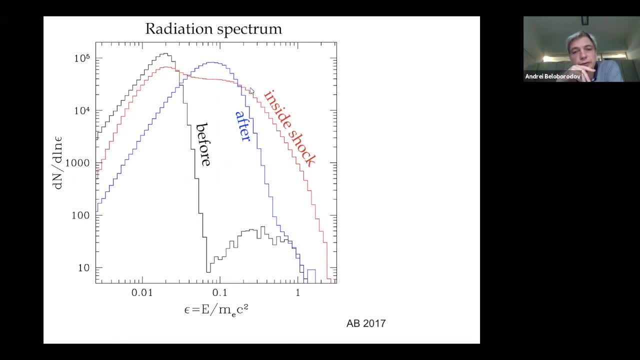 Fermi-like process. you have no thermal spectrum, So when this shock comes to the photosphere it will release something which is not quite thermal. okay, An interesting point here to make about the physics of sunshocks is that photons that reach energies above MC square. 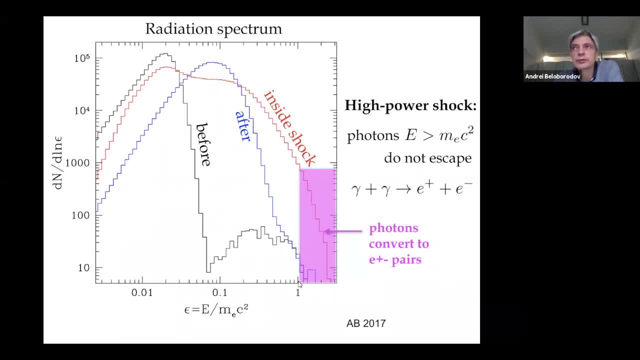 convert to pairs, Because we're talking about very energetic, high power shocks and optical turns out. optical depth of photon-photon collisions is much greater than one. So once photons come to the energy significantly above one, the energy is much greater than one. 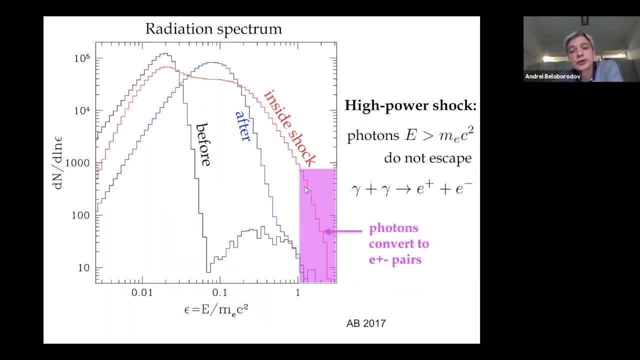 They convert to Now. as you see, there are not many photons in this region. only small fraction, like one thousandth of the total photon number, will end up above MC square. However, the number of photons is so big initially, like 10 to the fourth per barrier. 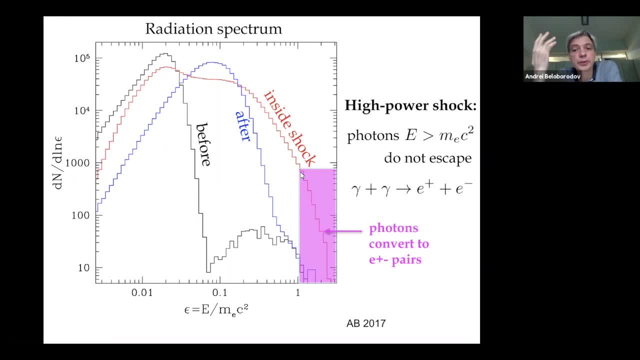 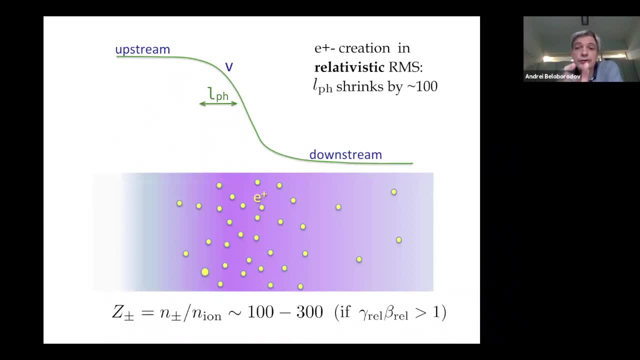 that you have a potential of creating a lot of pairs per barrier, okay, And your plasma becomes predominated And your shock shrinks. So in this simulation actually that I mentioned here is actually, number of photons per barrier was 10 to the five. 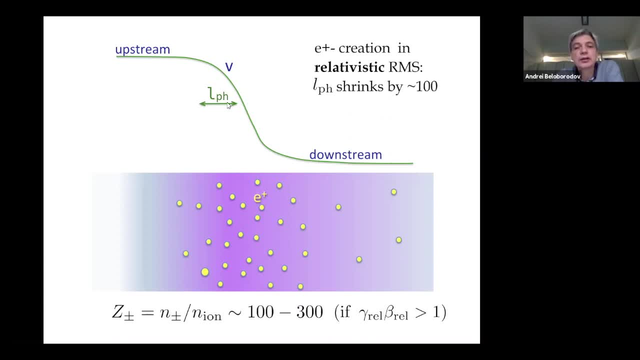 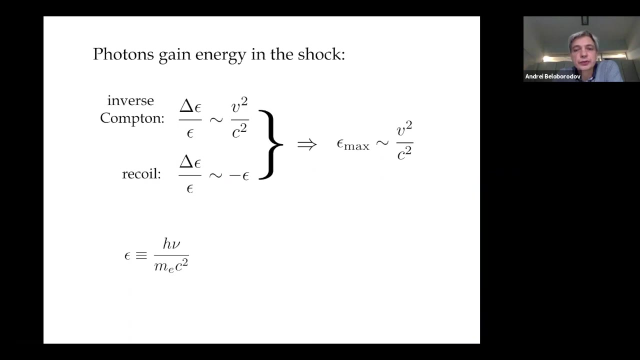 So the pair loading factor was actually a hundred, And then just you can see that the photon free path shrinks by a factor of a hundred and the shock becomes much thinner because of that. There is a threshold for this phenomenon to work, though. 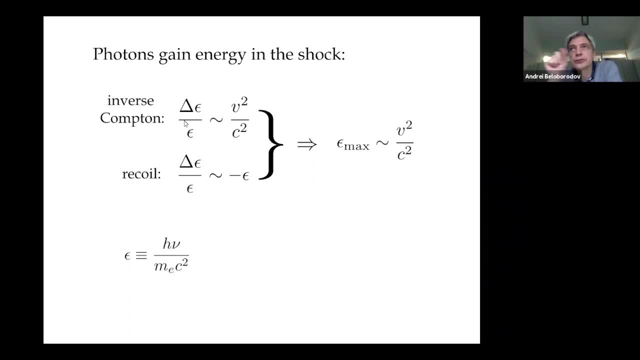 creation of pairs. Because when you look at how photons gain energy as they bounce between upstream and downstream of radiation-negated shock, on average in each bounce they get energy of four of V square over C square. The V is the relative force of this converging motion. 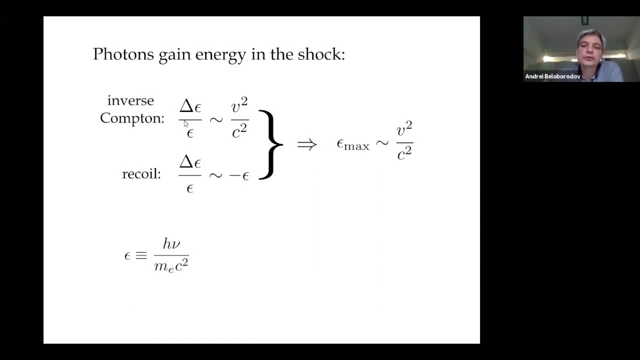 upstream and downstream. At the same time. photons lose energy. Delta epsilon over epsilon, It's the epsilon's energy, photon energy. so from C square electron resonance It's a four of negative epsilon Recoil Compton effect right. 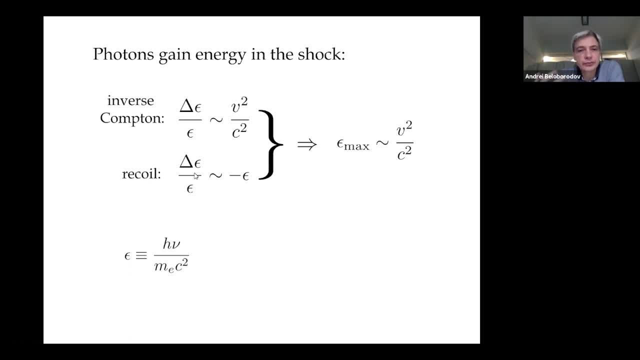 So shock can Comptonize photons, for normal relativistic shock only up to V square over C square, which is below unity, And therefore normal relativistic shocks don't produce pairs. Photons don't get the buffer in C square, But relativistic shocks do. 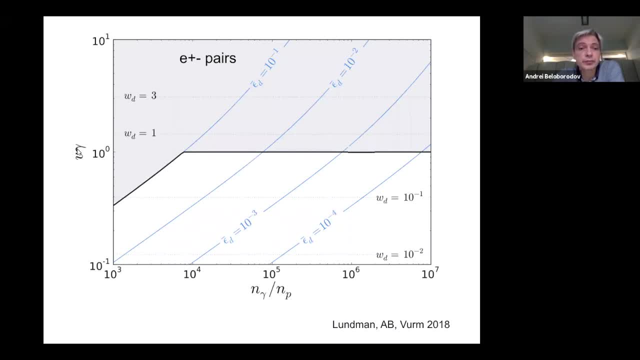 And the threshold for pair creation is basically better. gamma of the shock should be above unity Recall. we did many models. Christopher did many models. Christopher Verified that indeed there's clear separation. Shocks that have relative speeds above for the loss, above unity, produce a lot of pairs. 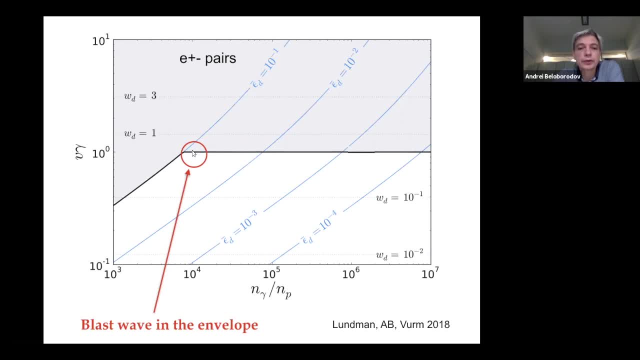 Okay, coming back to our merger, When you look at where it should be, at this, in this parameter range, it's actually right here, Actually a little bit below it turns out, And it does not produce a lot of pairs, But nevertheless we simulated it with complete Monte. 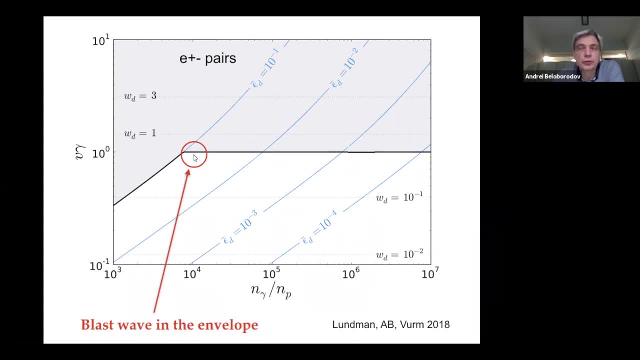 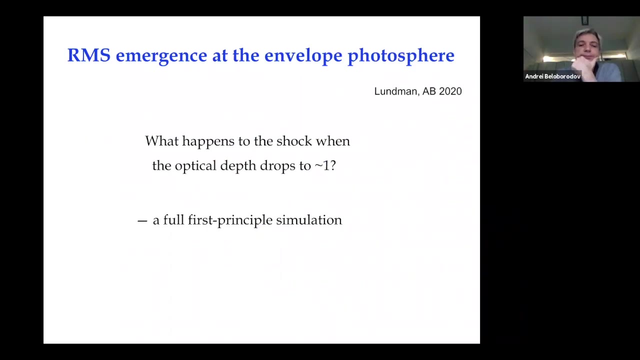 Monte Carlo code, which does follow all pair creation events And now also includes all the spherical expansion geometry. So basically we follow the shock as it approaches the photosphere And basically you want to see what happens. As a physicist, you would like to ask. 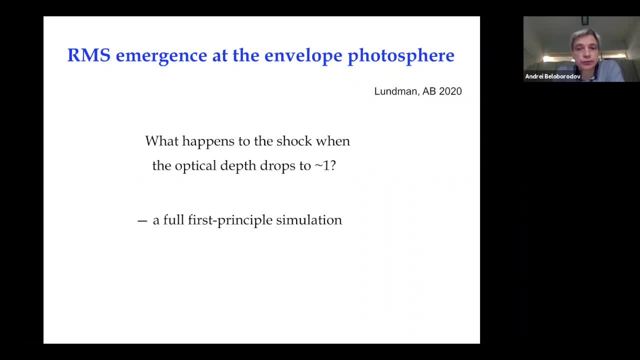 what happens to the shock when it come. when it comes to the photosphere, It should stop existing because the shock thicknesses- photo free part, But photo free but by definition of the photosphere- exceeds size of the system when you cross photosphere shock. 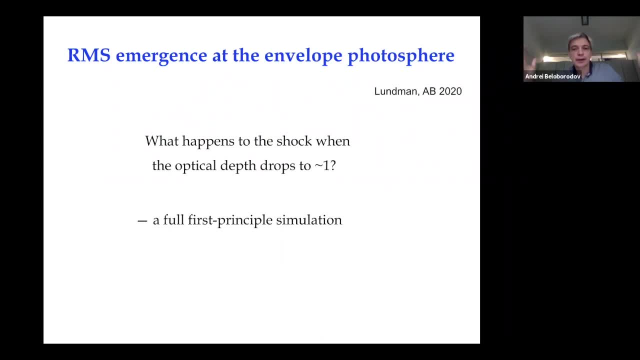 Radiation means shock is no longer supported, And so you want to understand where the energy goes. Okay, so it sits, most of radiation, but I guess it's tried to decouple from, from the plasma, and you want to understand what comes out. 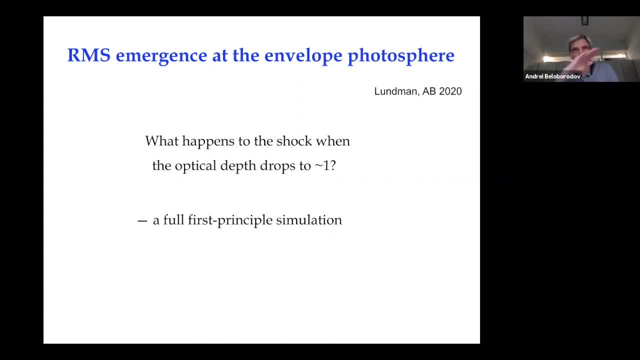 like probably you will launch. the velocity profile that was used to be regulated by radiation pressure now will steepen and form collision-less shock that you may expect As an observer. you would like to ask the question: what is emitted? What emission you should see? 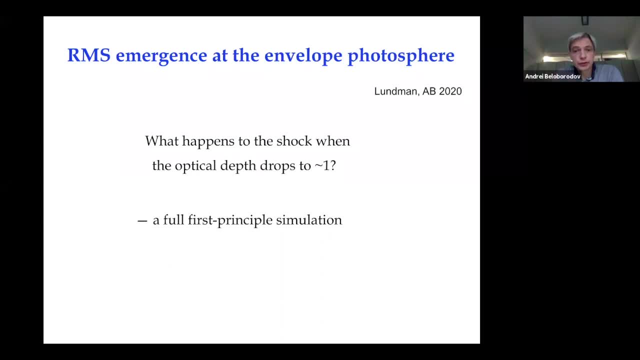 And so you need to follow this transition to collision-less shock in order to be able to predict what kind of emission of GRB this event should produce. The nice part of this problem is it's completely first principle problem By the time when you look at. 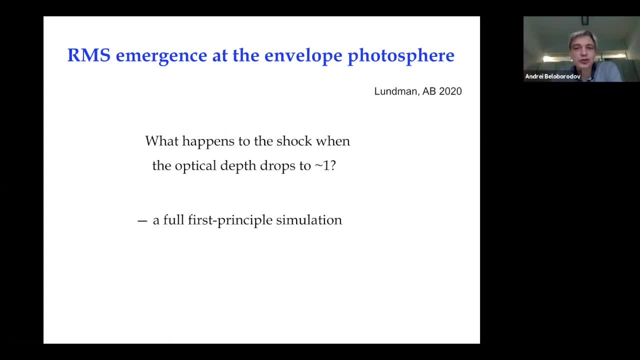 what is emitted by this blast wave? you can forget about the merger, the envelope, we just have a photosphere. Well, actually, stratification of upstream range factor is important, but that's it. you launch a shock. you see what kind of spectrum it produces? 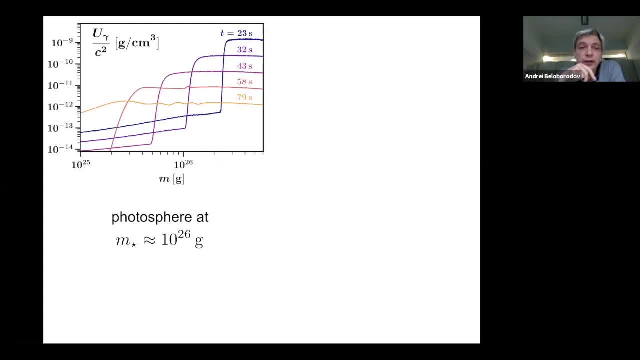 So we've done this simulation and you see here. so I have just a couple more slides to show the results. So this plot shows energy density of radiation different times. 23 seconds is not observed in slug frame time. basically radius divided by C. 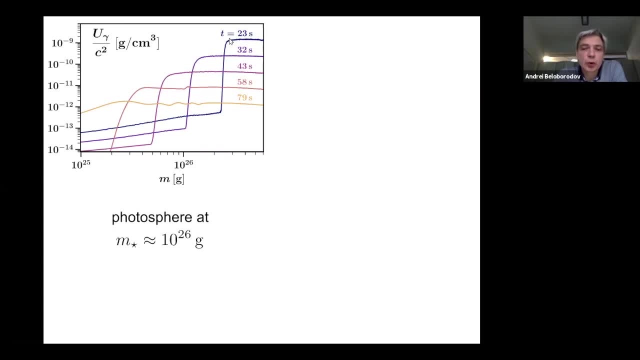 The shock approach is 10 to the 12 centimeters where optical depth drops to unity at about 30, so 23 seconds. So 23 seconds the shock is still below the photosphere and at later time it moves to lower masses right. 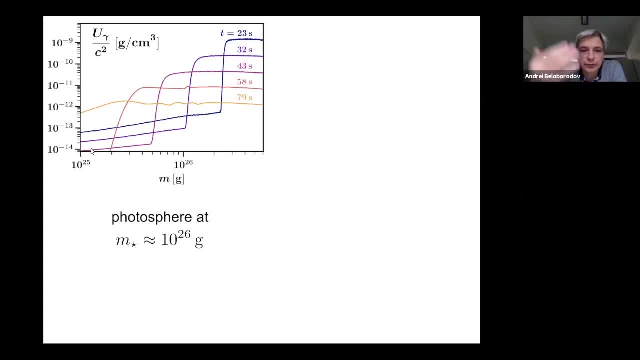 To the outward, in other words, masses counted from outside, And then, okay, radiation keeps moving, okay, So we don't see anything from right here. but when you look at the profile of gamma-beta, that's how it transforms. 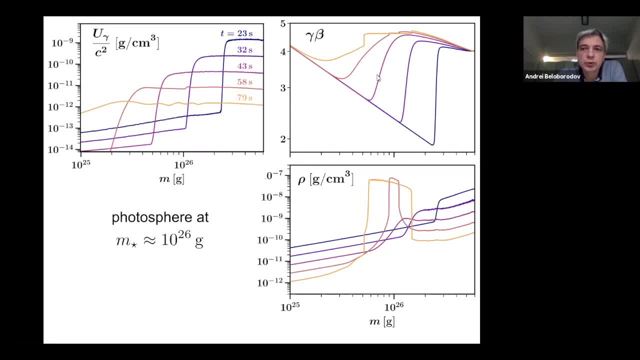 That's the pre-photospheric shock. it becomes broader and shallower, okay, And what you see here is the formation of a pair of two shocks. This is one collision-less shock- forward shock- and there is a reverse, collision-less shock. 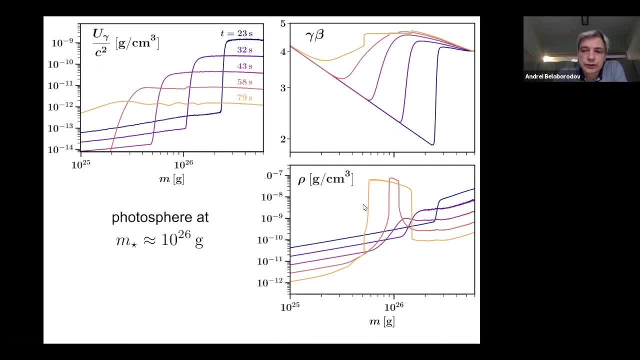 So the mechanism for formation of a pair of this shock, like this transition from radiation-mediated for two collision-less shocks, is actually straightforward. The plasma, the motion that used to be regulated by radiation pressure, suddenly feels like radiation pressure is not telling it too much. 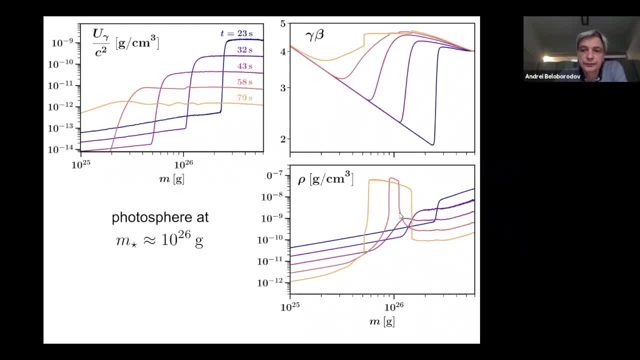 and it just continues to move ballistically And the profile of velocity continues to steepen and you form a caustic. So when you look at the density plot- here it's the three panel- you see how what used to be one 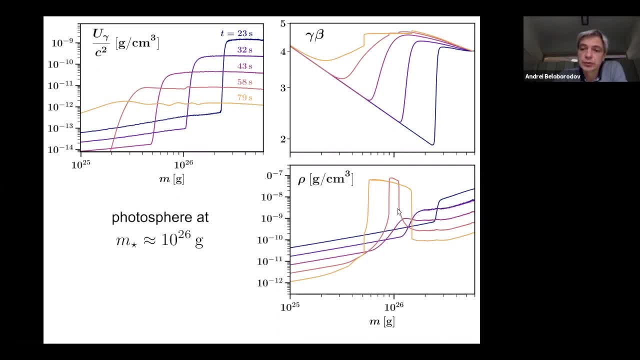 that's the short profile, the second snapshot. At the next snapshot you see how density shoots up at the position of the caustic. So you have a very thin layer that keeps compressing until the density increases by more than a thousand. 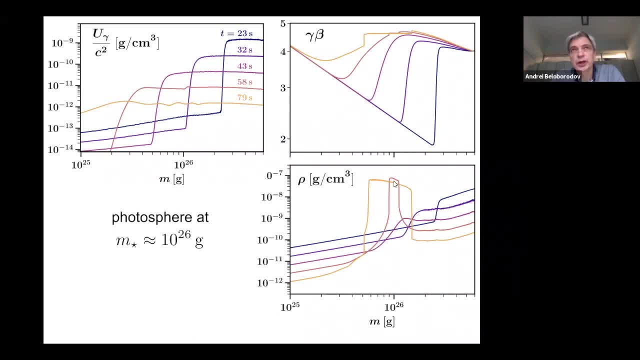 And at that point the gas pressure- now with radiation pressure, gas pressure- balances the run pressure in the shock And at this point it stops the compression and you launch a pair of now collision-less plasma-mediated shocks forward and reverse. Okay, that's the basic physics effect that works here. 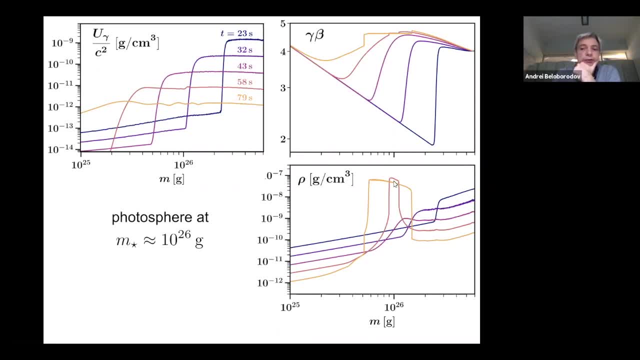 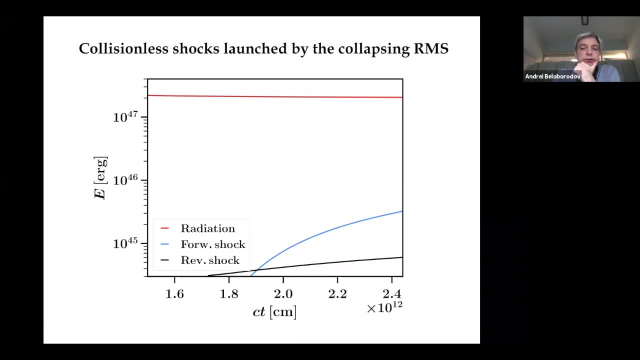 And it's really interesting. but then you can ask for that problem how much energy you deposit into this collision-less shocks, And actually it's something that we did not expect. but when you calculate this energy, you find it's almost nothing. 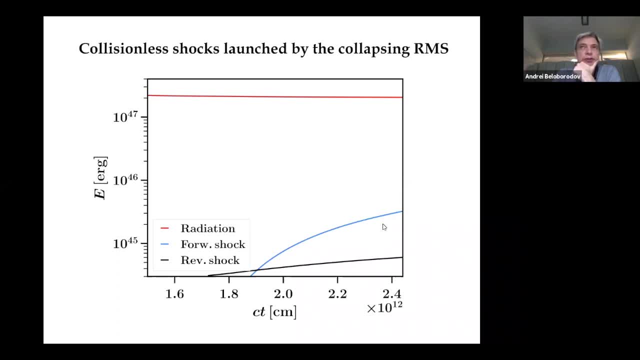 It's like 1%, And so basically the first approximation. what happens in this radiation-mediated shock breakout is that radiation peacefully decouples- and yeah, there is some leftover plasma motion, but it's mostly peacefully decouples- photons just leak out. 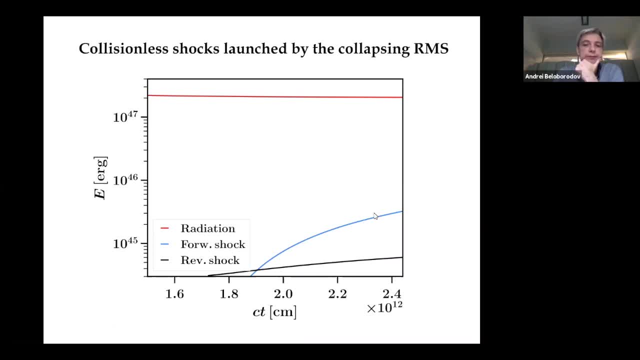 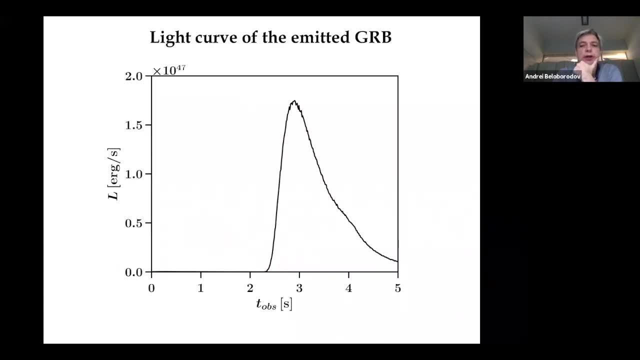 and whatever energy they've got, they deliver to the observer. that's it. Peer creation is not triggered. We see in our simulation there's some peer creation, but it's negligible And to show the light curve. of course it's a Monte Carlo simulation. 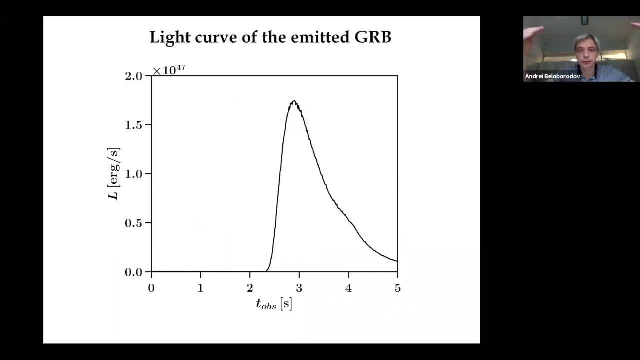 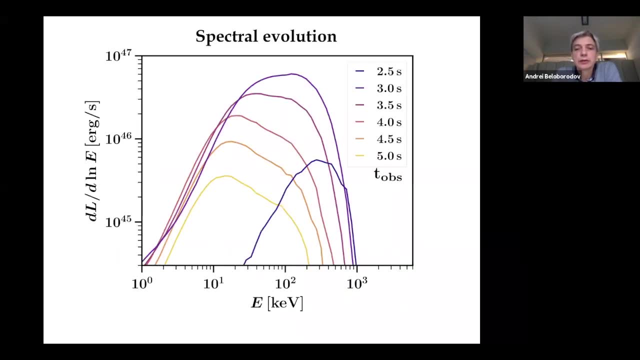 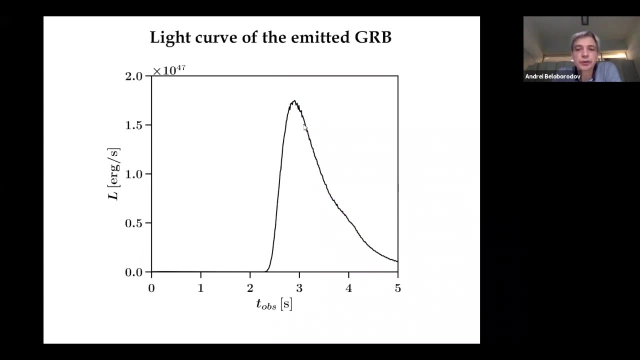 so we see photons, what they do individually, and we collect them at infinity. this is the light curve from that explosion And this is the spectral evolution. So the light curve has a delay. duration and luminosity as expected. Delay is actually a little too big. 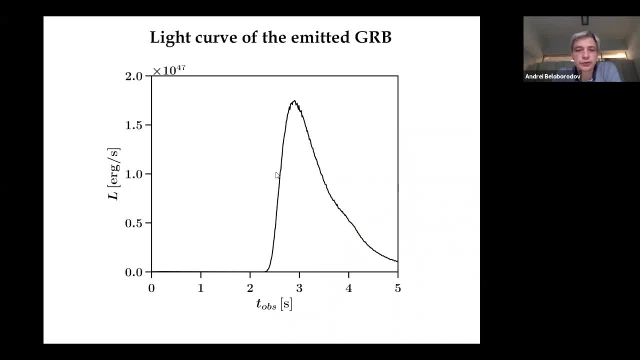 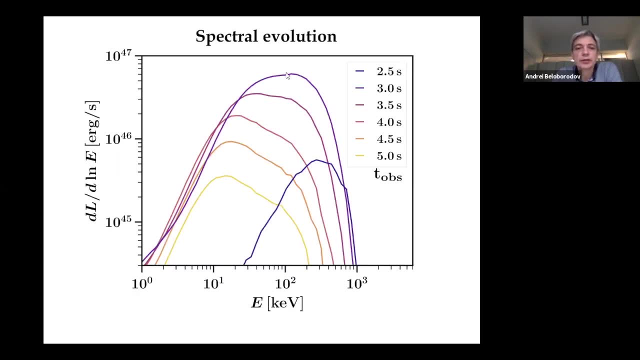 but it's because we chose the delay which is now we're running it, making it a little short. It will not change anything, except it will be at least two seconds, And this is the spectral evolution. So you start with very hard emission. 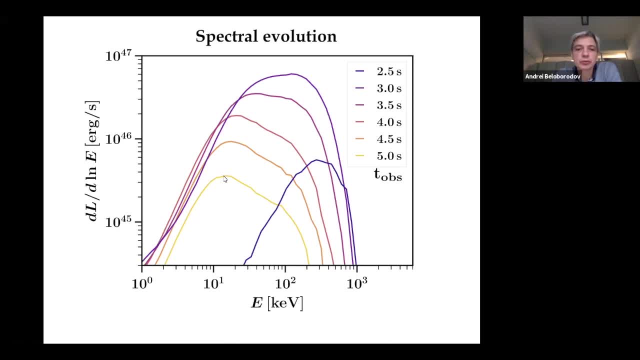 and after a few seconds it comes to basically a 10, 20 key spectrum is observed. So the bottom line is that this blast wave seems to give you the observed therapy just from first principles. and wouldn't they pursue activation? 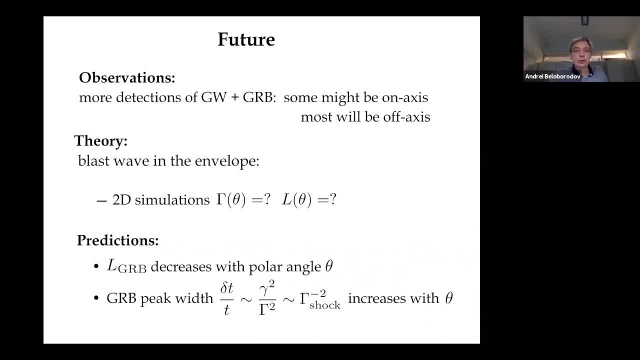 And I should. I guess I should stop now. yeah, So this is like slide. talking about future, The most interesting part, I think, theory to do is to do two-dimensional simulations and try to make predictions For future when you look at them at different angles. 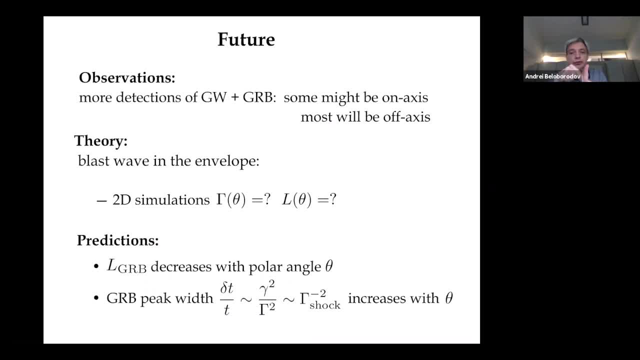 then you expect different luminosity, different Lorentz factory, different duration of the peak. If this mechanism is indeed at work for off-axis GRBs, for Newton's time murders, then it's pretty much the same for murders, except for the viewing angle. 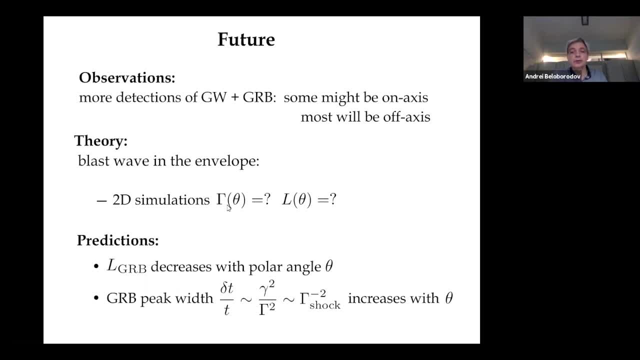 And you can make predictions for correlations between, let's say, luminosity and delta T over T, for example. It should increase with that, while luminosity should grow with that. And I'll stop with this point. I'm already a little late. 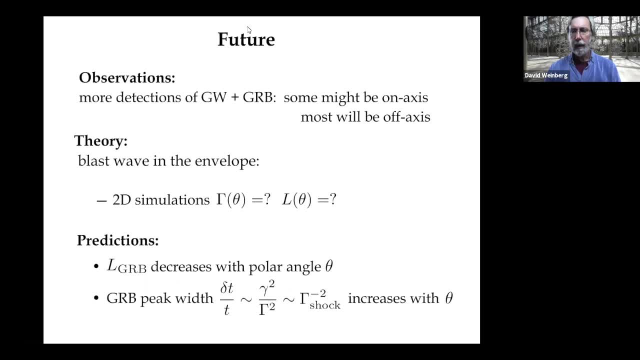 Thank you, Great thank you, And so we have time for a few more questions and then, if you wanna go dive in further, can join this afternoon's conversation. If you have a question, why don't you use the Zoom? Zoom raise hand. 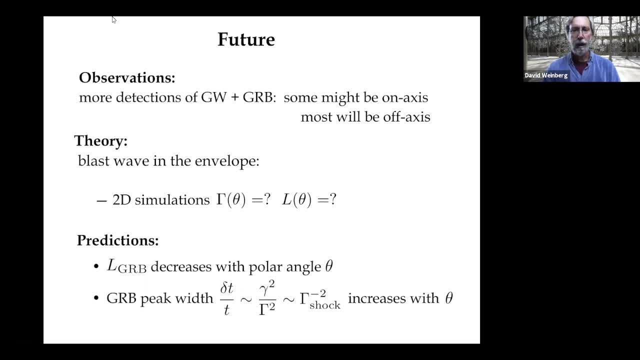 so I'll try to make sure everybody gets their questions in. I guess a question I had was: are there, have there been, any other, at least semi-viable, proposals for explaining this gamma ray burst? I mean, the story you've told here seems pretty compelling. 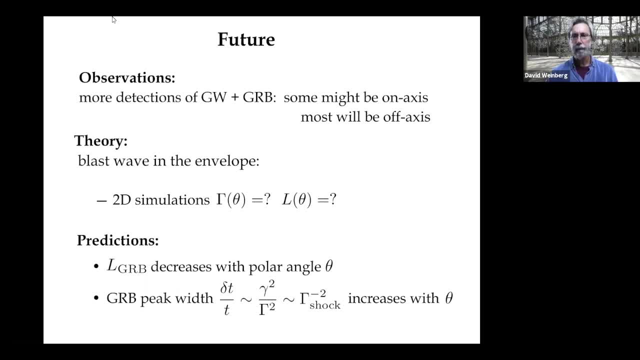 but what are the alternatives? So what was discussed? So there are basically two existing proposals, my knowledge. So one is short breakout. This is what I discussed in detail And I think this is the version of the process that works Now. the other option is the emission from the jet. 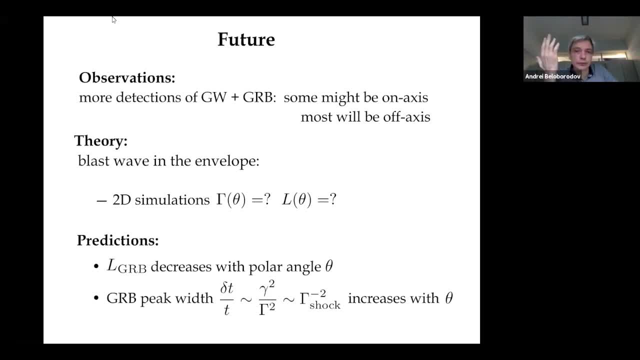 itself, not from the blast wave that was launched in an envelope, but from the jet itself. It's similar to canonical GRBs that we observed on axis And I think when you look at the same exposure on axis, you will see very collimated jet directed toward you. 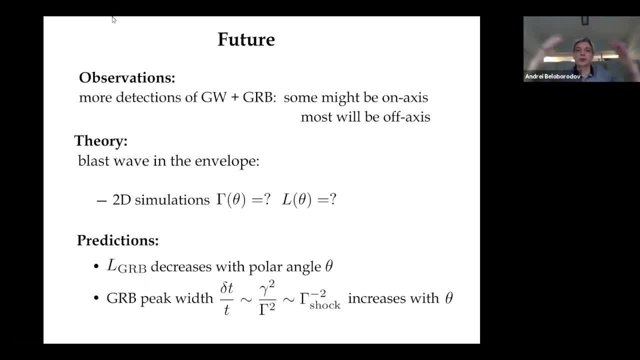 which would be so bright it completely overshadowed whatever side wave, last wave you may think about on axis, And in that case you would probably look in directly into the jet and some dissipative process that works inside this magnetized material in the jet. 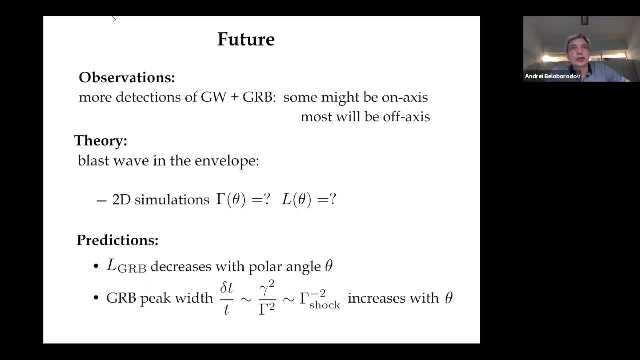 So in principle you could tweak the jet model, but it's hard to do. Like, for example, if you say one proposal that was initially discussed and ruled out most immediately is that you look at your gamma ray, is the gamma reverse? 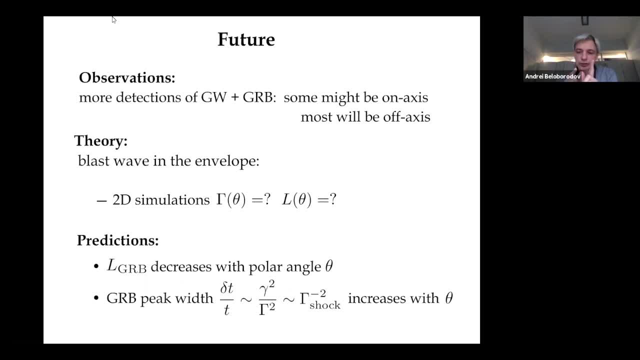 is the gamma ray emission from of axis narrow jet And it turns out that it's in peak position. spectrum peak and luminosity are not consistent with that idea. Or you could imagine a jet which is kind of a structure jet where we're inspecting luminosity. 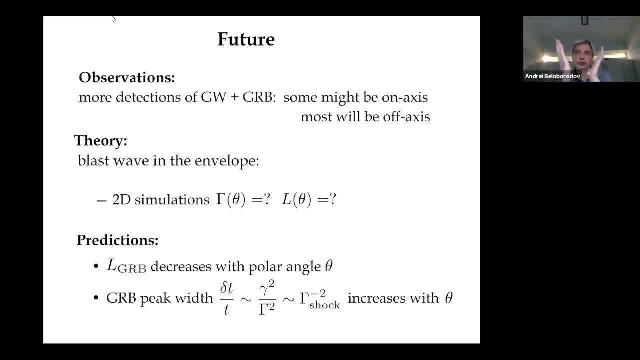 you can draw a function, try to adjust it So that produces the luminosity that. you see The problem with that. so it's hard to calculate from first principles. So you can try to, but in my mind and actually it was always the problem known. 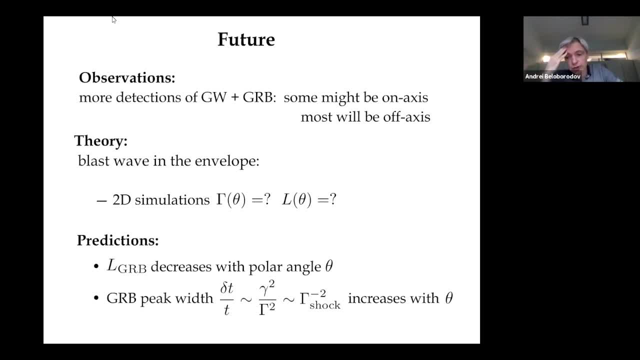 before the discovery of the burst is that these sources are typically soft X-ray sources or hard X-ray. there's no gamma ray sources. That's yeah. Thanks, Elias. Right, I basically wanted to ask again about this 2D dependence. 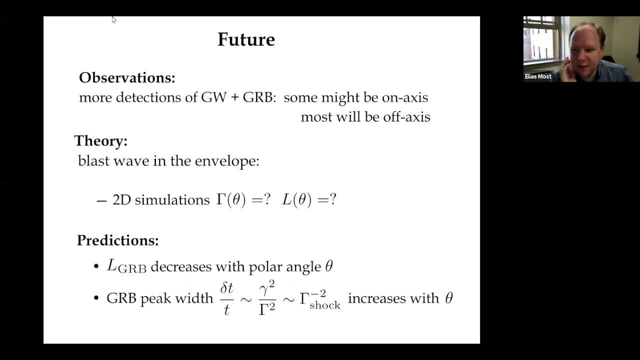 because, if I remember, like your comparison with the theory and the observations, you basically got something that was more like gamma is three versus gamma is five, Like, do you think this is really just by you know the angle you look at this? 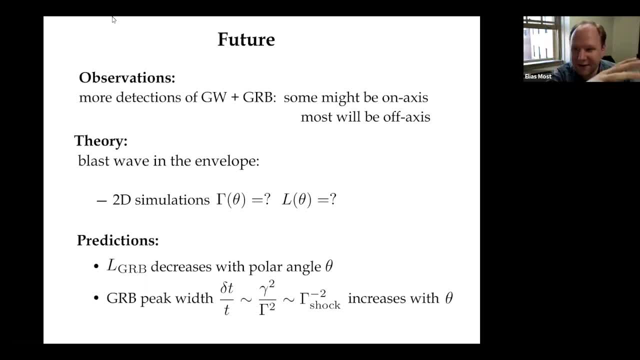 or is this because, I mean, in your model, even this envelope should have some angular dependence, right? if you really think this comes just from you know this ablation, this would not be homogeneous. So what are your thoughts on that? 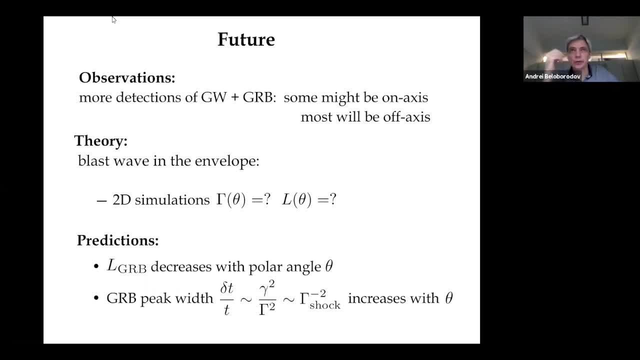 I think the main factor is simply the power of the blast rate, The envelope. it's not exactly spherical, symmetric for sure, but it should be quasi-spherical, at least at the range of angles of interest. But the blast wave is strongly in androgynous. 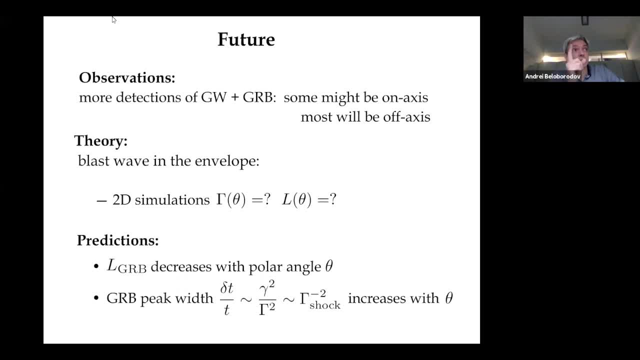 because the jet is so much correlated And so basically, when you look at a small angle, there is more power. This capital gamma is higher, essentially. I mean because you push with, the piston is bigger And when you go to lower theta. 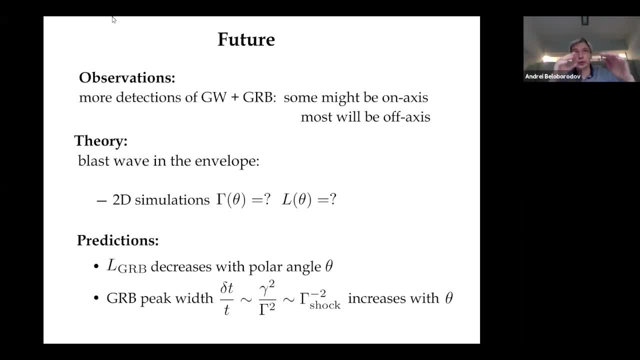 you come to this situation where it's capable, And so you can draw a photosphere at different angles. The blast wave comes to the photos for a different gradient, And so that's how you can make predictions. You take a simple small, the spherical envelope in an entropy blast wave. 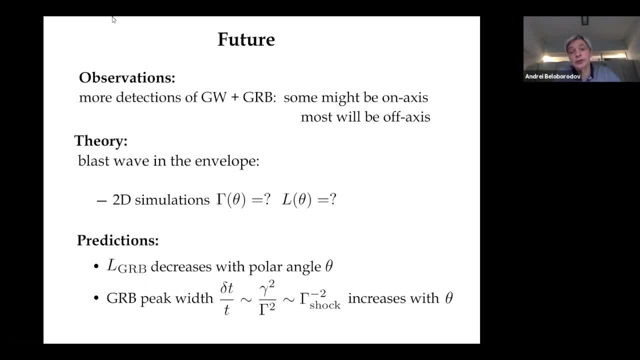 and see how things depend on that. That's what we were trying to do Hygienically. it turns out to your presence, maybe I don't know. it's kind of a nightmare. It's kind of an optimistic two-dimensional hydrodynamics, but hopefully it's all over. 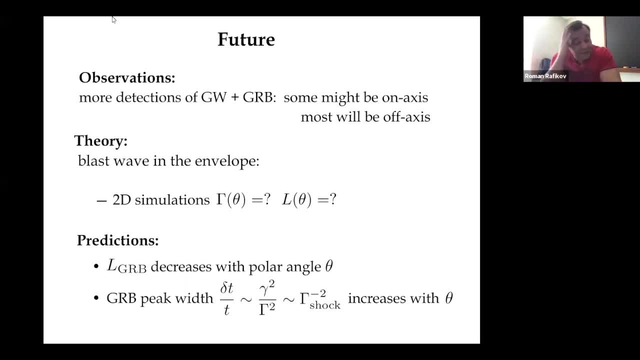 Okay, Roman, you get the last question. So, Andrey, it sounds like I mean, what you're sort of proposing here is different from the canonical model for the production of GRBs, at least this is my impression. So then I mean: so does it mean that this explosion? 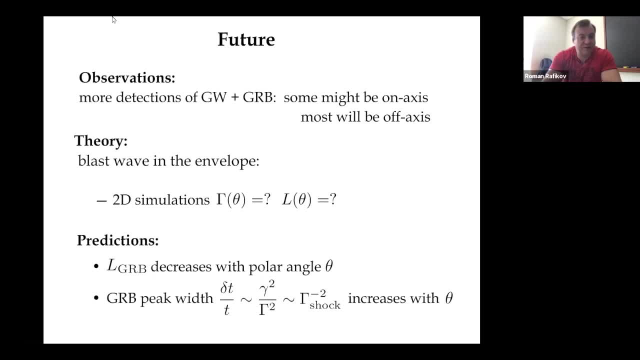 was in some ways special, And if so, then why? these? these physics that we described here does not work in the regular GRBs, So the key difference is the angle. So- Yeah, but I mean, if you do observe many GRBs? 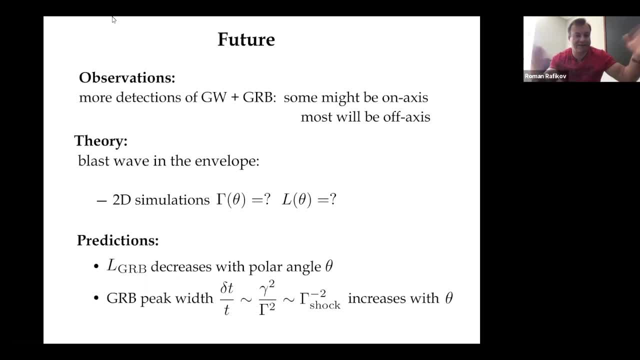 I mean, why don't we observe many GRBs that are just slightly off axis And see these- Ah, it's weak, That's right why? Because it's- You just don't pay attention to it. You just say that this is not a real GRB. 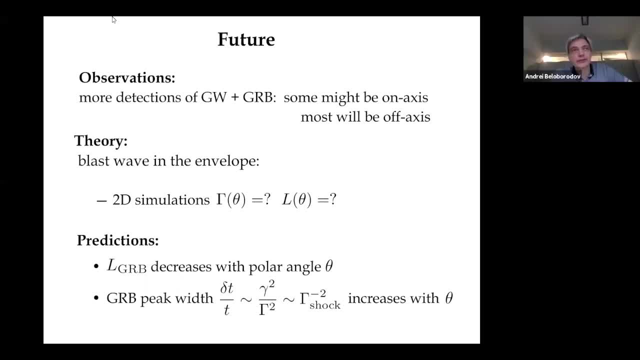 this is some noise of flukes and so on. Yeah, so think of it if you. how many? how many times? how many times do you do this? Yeah, so think of it if you. how many times do you do this? 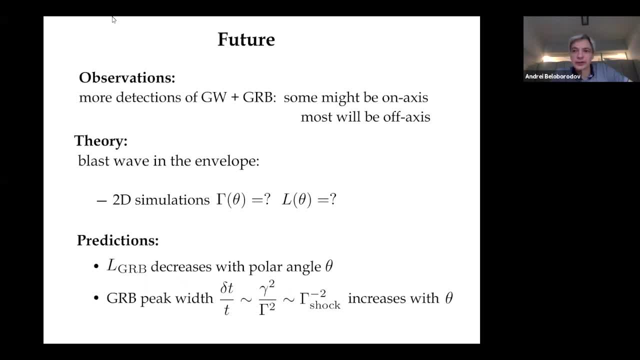 sources with luminosity 10 to the 47 earth per second, lasting a second, you would detect. i have no idea. i mean, you're an expert. yeah, yeah, so it's, it's. it's hard to to detect uh of axis. so you, when you look at the in the sky and you collect gamma ray bursts from the sky, what you 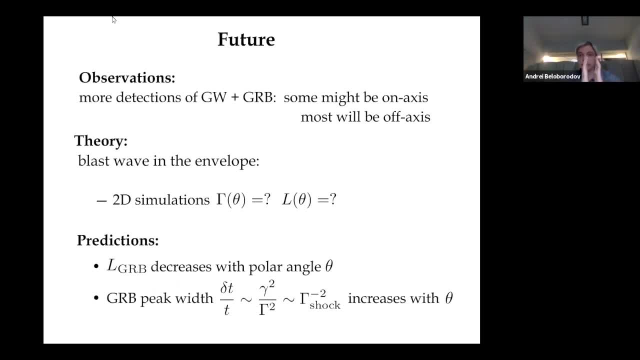 see are more distance, but really more distant, but really well collimated towards you- bright sources- and they have different physics because you look right head-on into the jet and i think for those sources as well, if you had a chance to look at the off-axis and you are close enough to detect. 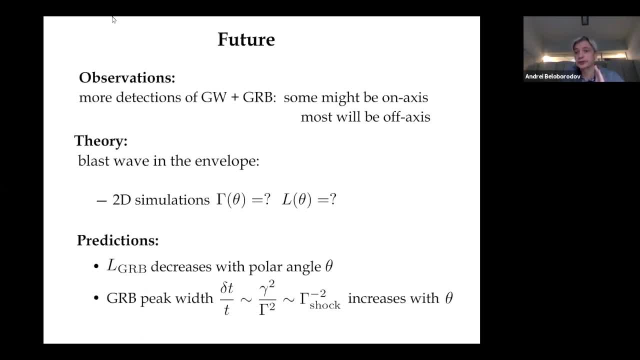 it easily. this will. this person was marginally detected, but the distance was already 40 mega parsecs, so it's really it's hard to detect from large distances. this is not strong first, but if you looked at them at 20 degrees, i think you should see something like that in this picture at least. 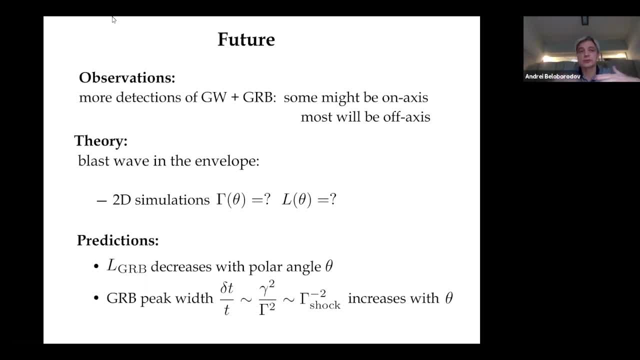 something you should see: a sideway blast wave from the jet which would propagate into the ejector from the merger and i think it is enshrouded with so similar dark and low and it will come to the photosphere and produce something. so we should see this generically as we detect more neutron. 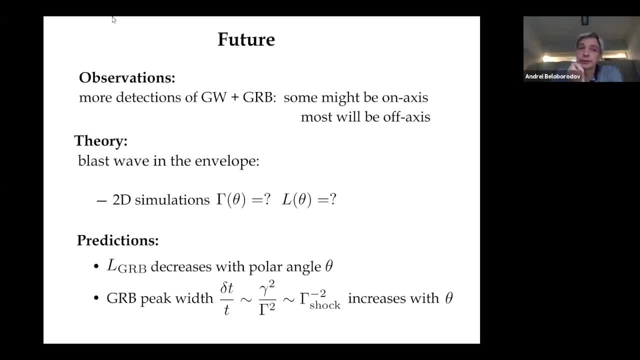 star mergers gravitationally. absolutely, yeah, hopefully, yeah, okay, well, thanks, uh, let's thank uh andre for a terrific talk towards uh, all sorts of fascinating stuff in there, and so thanks so much, and um and uh, those who want to join again uh this afternoon, and thank you again for for joining us and and giving us. 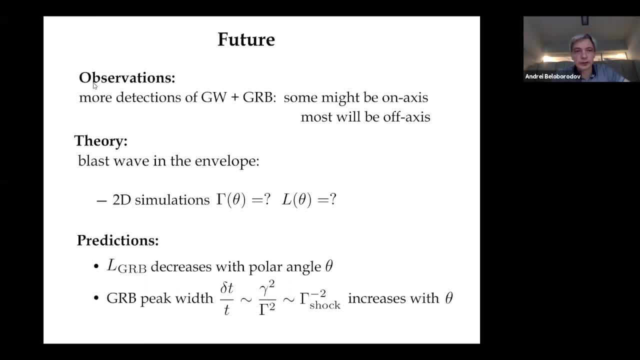 that presentation, the three same link. right, yes, same link. okay, okay, bye.